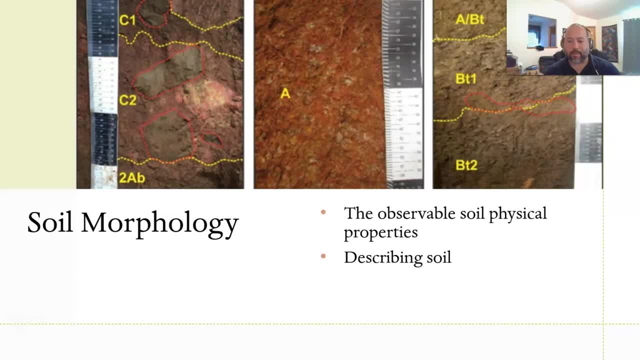 that we're now going to look at those physical properties, We're going to observe them and we're going to describe them. So we're going to now try and see those in the soil and see where we can see the differences, And then that's going to help us describe the soil even more. And so if we take 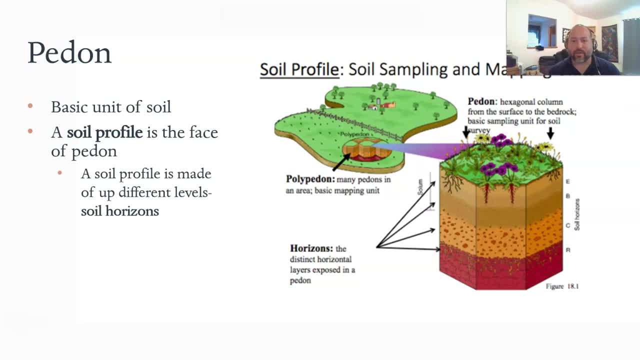 that down to A basic level. So if we look at anywhere, any place where we're looking at soil, our basic soil unit is going to be a pedon, which is this hexagonal column all the way from the top, which is the. 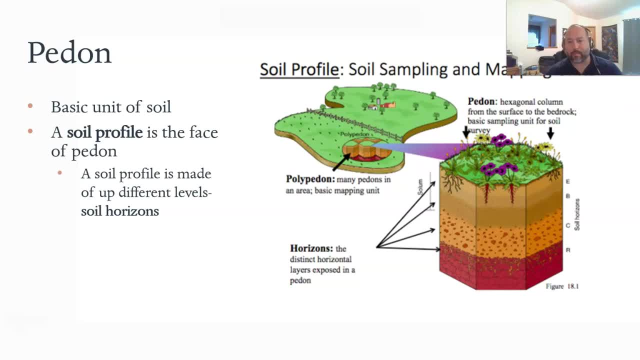 surface all the way down to the bedrock, And if you have a bunch of pedons together, that would be a polypedon, where you've got many pedons in an area, And a polypedon is when we put together like a soil. 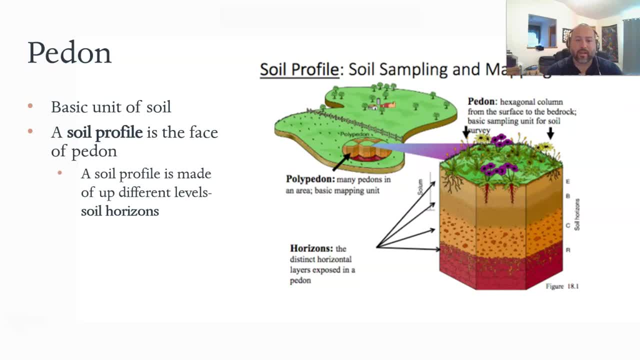 map. that would be your basic map, A soil profile. when we come up with a soil profile- or we looked at soil profiles- what we're really just looking at is one face of a pedon, whether it's here or here or here. we're just going to look at the changes in the soil within that one face. 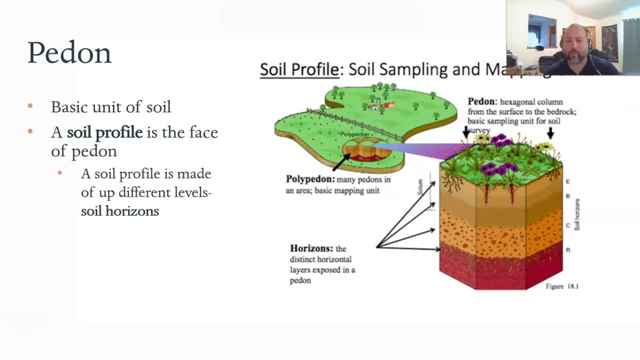 And then so within a soil profile you have horizons, and horizons are just the different layers within that soil profile. So if I pick one specific base here which is right here, we can see that there's a layer here, another layer there, another layer there, another layer there. 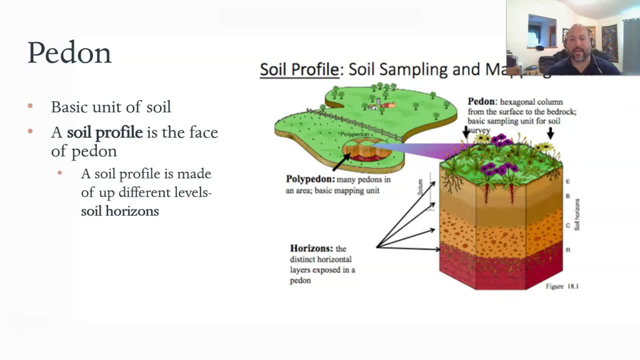 And then we're down into the bedrock, And so that's what we're really kind of talking about today. We're just going to try and see how we- how we would describe this- describe a pedon and a soil profile and all the different terminology we can come up with. 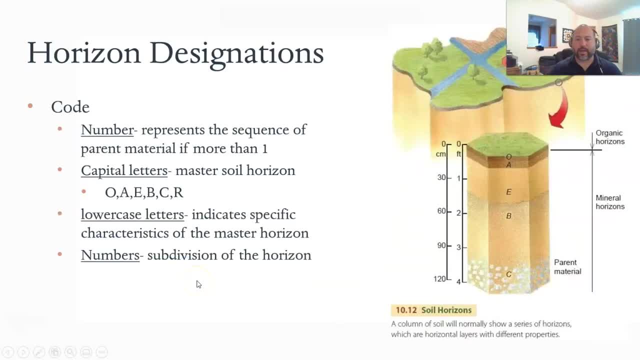 So let's take a look. So, in order to describe our horizons, our different soil layers, they've come up with a coding system. So it's a number: a capital letter, lowercase letter and then a number. Now, not every one of, not every layer is going to need all four of those. 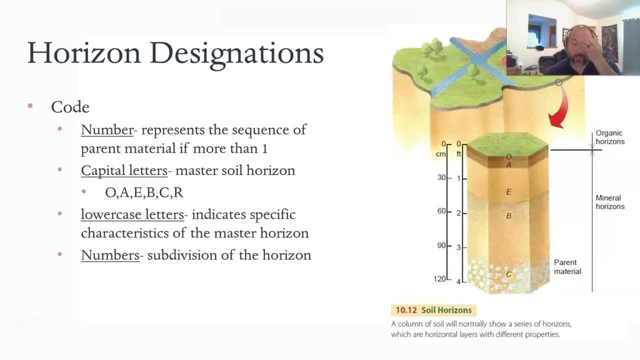 Some of them might use all four of them, Some of them might only use three of them or two of them, But it just kind of depends on what is present in In that layer, because it's trying to be- we're trying to be- as specific as we can without being as complicated as we can. 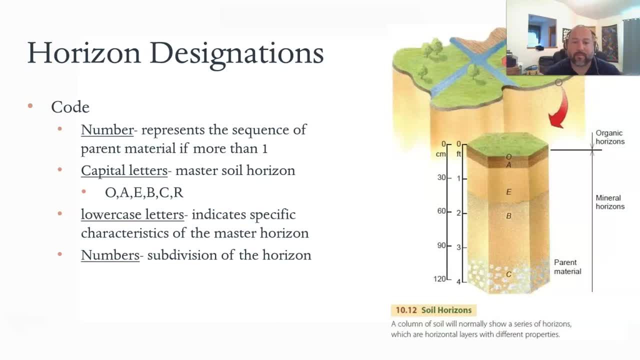 And so the first number would represent the sequence of parent material, if there's more than one. So what does that mean? It means that, if there, if it formed from two different parent materials, like you, had, you know, a natural process. that's happened for a long amount of time, and then something else happened as well: that you get soil forming from two different parent materials. 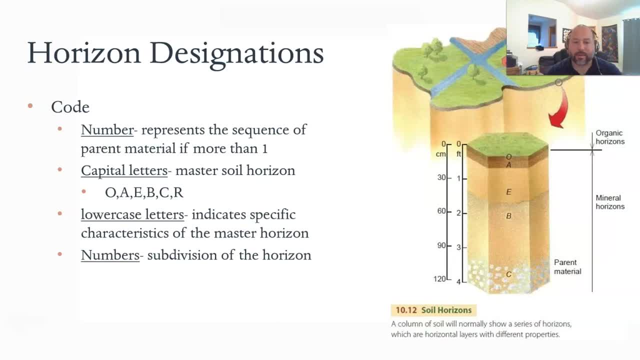 Then That number would represent the different parent materials. Usually, though, that's not, that's not a super common thing, So you don't really see that first number in a lot of soils, But usually the first thing you see is a capital letter, which we can see here in this example right here, where we see the O, A, E, B, C for for these different layers. 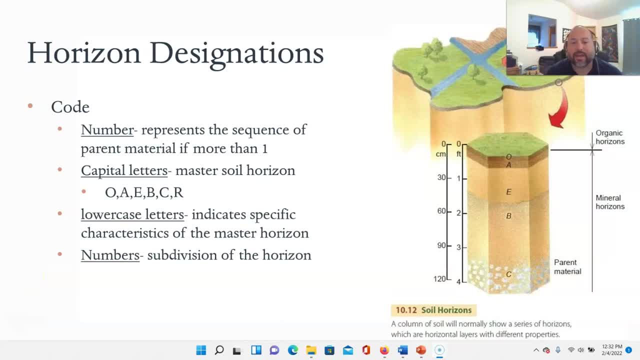 The lowercase letters that then follow the capital letters are going to indicate specific characters, Characteristics of the master horizon. So our capital layers here, those are our master horizons. in this one Specifically, we've got our organic layer, our topsoil layer, our leaching layer, our subsoil and our parent material. 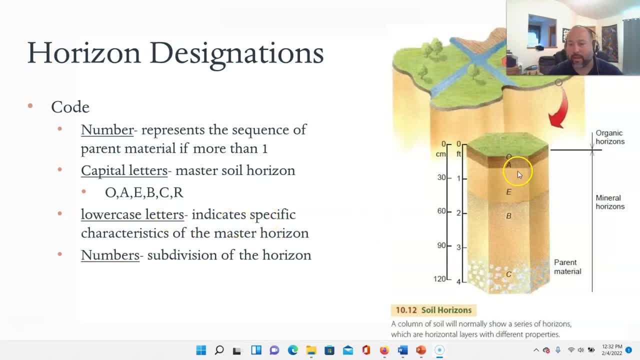 And we'll go over all those in detail. But then there'd be lowercase letters after it. One that's common is you can see an AP for your topsoil And that just means that it's been. it's the layer that's been plowed after the lowercase. 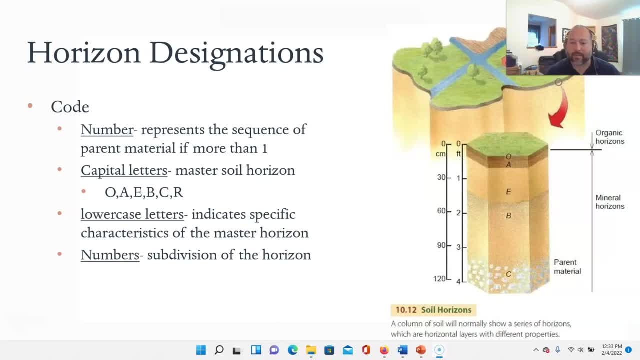 Letters. You could then have numbers again, which would be subdivisions of the horizon. So if you, if there's some sort of a reason to say that this part of the, this part of the horizon is different from this part of the horizon, but it's not a completely different horizon, then we would use the number system to to separate those. 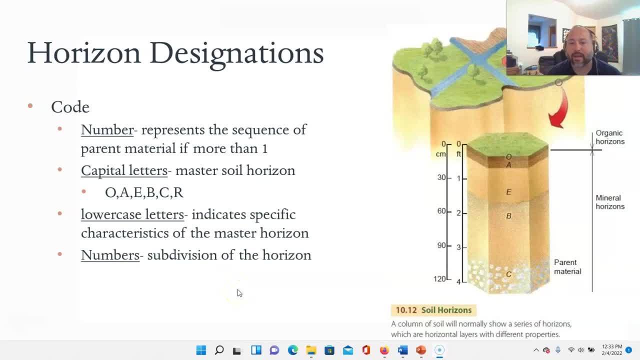 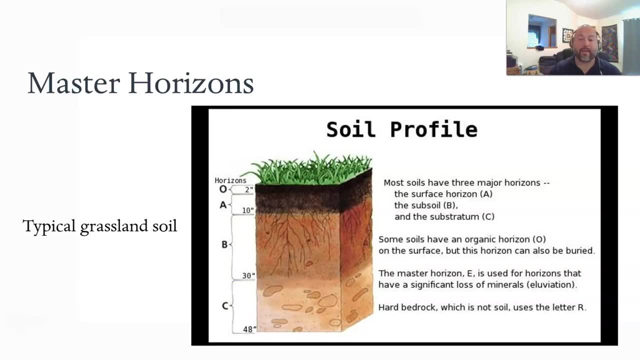 But we'll kind of show some examples and do our best to kind of make that understandable. So what we'll do is we'll take a look at at a typical grassland soil, but we're also going to throw a forest soil in there just to kind of give us a look at the at the soil profile and the different master horizons and why, why they're different. 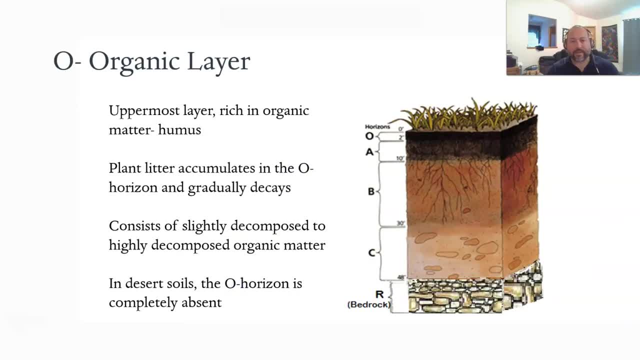 So the first one we'll start off with is the organic layer, which is at the top. Now, the organic layer is not always at the top, So the way I like to describe this to people, To hopefully not get them confused, is that this order that we see them in, with the horizons, the O, A, B, C, R for this typical grassland soil. 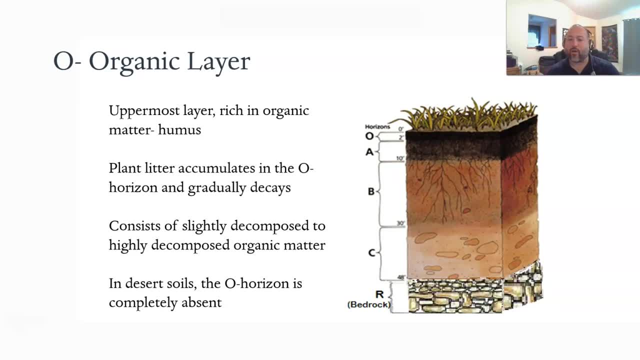 That's the order that it has to be in if all those layers are present. However, you don't have to have all those layers present. What do I mean by that? Well, you don't have to have an O layer. For example, if it's a desert soil, you don't have an O layer. 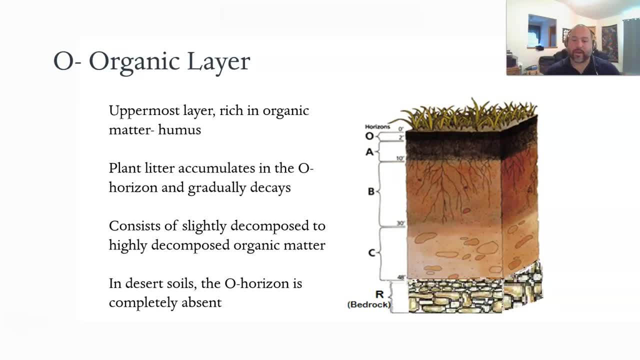 Why? Because there's nothing, There's not a lot of stuff, And the desert, to create that surface, litter that then becomes humus, that then works its way into the topsoil, So you don't really have an O layer in the desert. 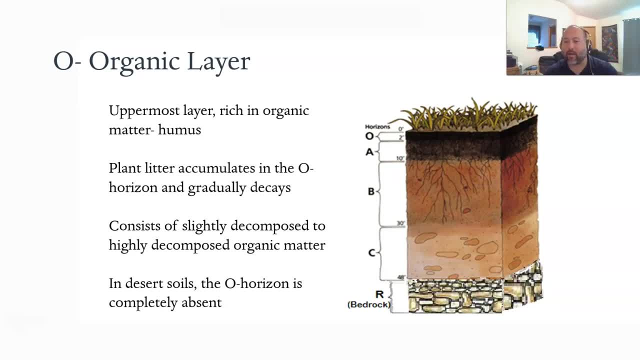 So it would just start A, A, B, C, R and go from there Or down in the Kern River. there is no A layer or a B layer. It starts off as a C layer And so you start off right at C, down down at the perimeter. because it's a, it's been formed by alluvium. 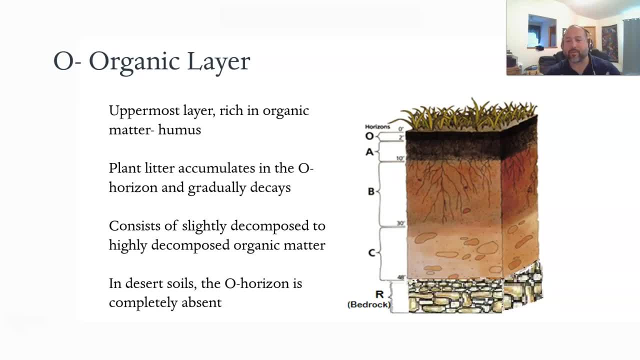 So stuff is constantly washing in and out, So you don't really have any topsoil or subsoil development, because when the water is flowing all that stuff just kind of washes away. And so that's the way to kind of think about it, that there is an order to these things, but not every layer has to be there every single time. 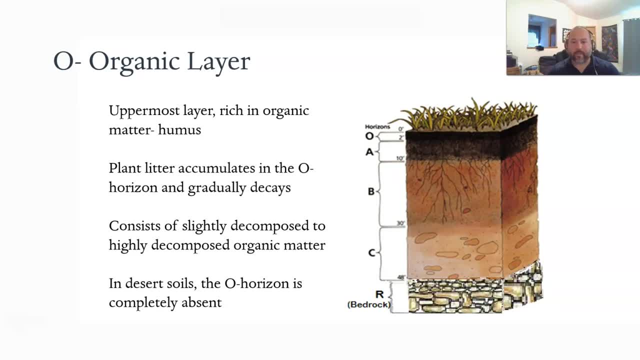 And so if we're starting off here at the organic layer, we're actually talking about the surface, the surface litter and the organic material that's working its way down From the top. that's why the next layer is going to be called the topsoil, even though we've got this organic layer over the top of it, because the topsoil is the top of the soil working its way up, because everything started as rock down there in bedrock. 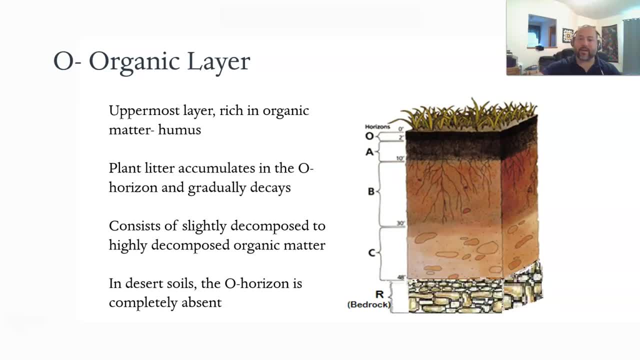 Then it became weathered bedrock, which is that C layer. Then it became soil. that became layer after layer after layer after layer until we got to the topsoil, And then the organic layer is the stuff from the surface that's working its way down into the soil. 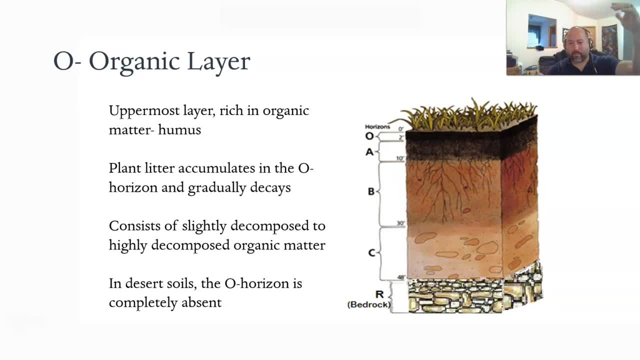 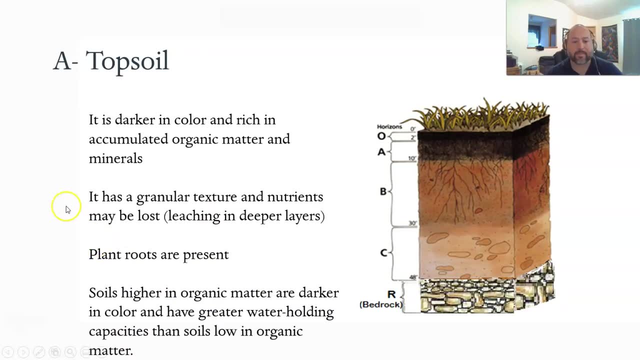 So the organic layer is on top, taking things from the surface and bringing them into the soil, And then our next layer is our topsoil, which is the top of the soil working its way up from the bedrock. So the topsoil is usually darker in color and that signifies a richness of accumulated organic matter and minerals. 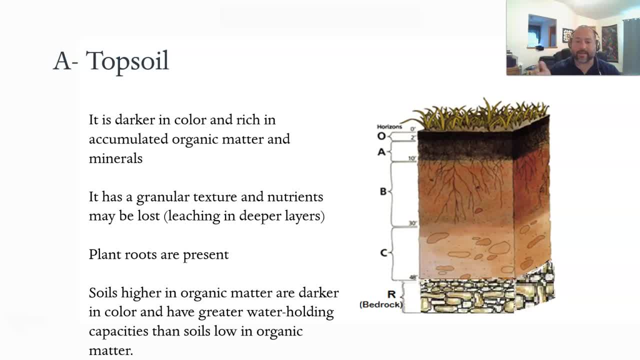 And also if your layers, If your soil is nice and healthy and everything's going right. your soil should go from darker to lighter as you go along, because you have this greater presence of organic matter and minerals, because it's working its way from the surface down. 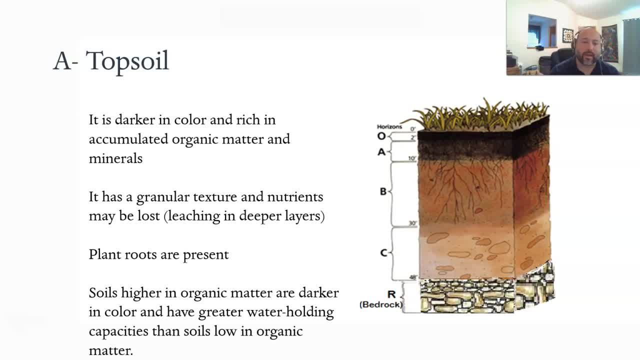 And eventually you're just going to have less and less as it works its way through the soil. Usually the topsoil has a granular texture and nutrients will be leached into the deeper layers. But you know, a lot of it's going to. 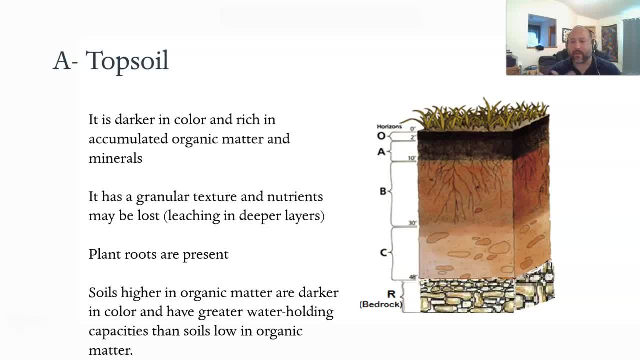 Get used up there in the topsoil. That's why the topsoil is so rich, That's why we plant, and most of the roots and everything is just in the topsoil And it doesn't really go a lot deeper than that, because that's where it basically the topsoil provides the plant with everything that it needs. 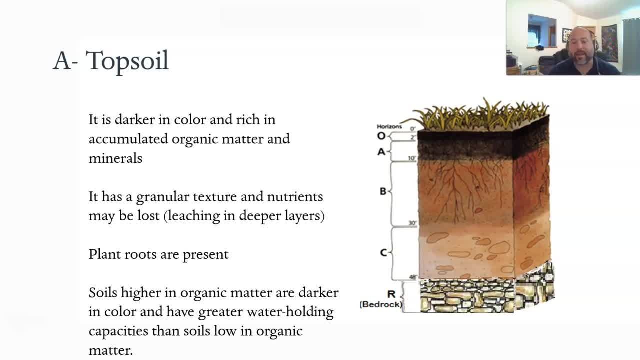 So definitely a high presence of plant roots. Soils that are higher in organic matter are usually darker in color and will have a greater water holding capacity. That's one of the great things about high emissions. The amount of organic matter is they can hold on to water really well, which is great. 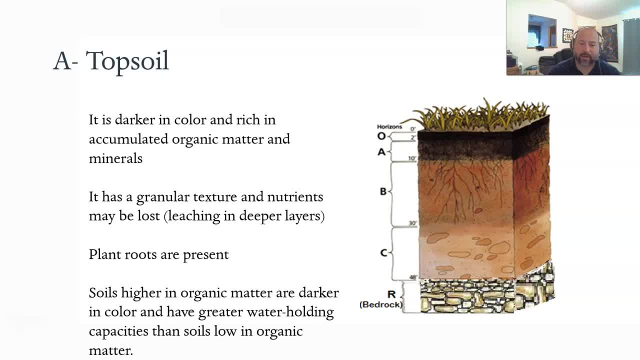 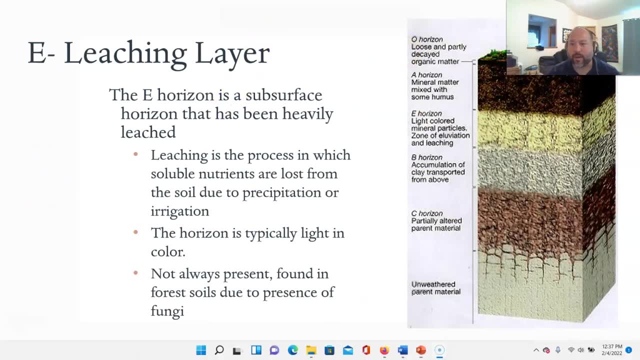 If we see lighter colored soils, less organic matter, less water holding capacity. So here's where we switch into a forest soil and I'm going to move myself over here so that I'm not Oops. There we go. That's better. 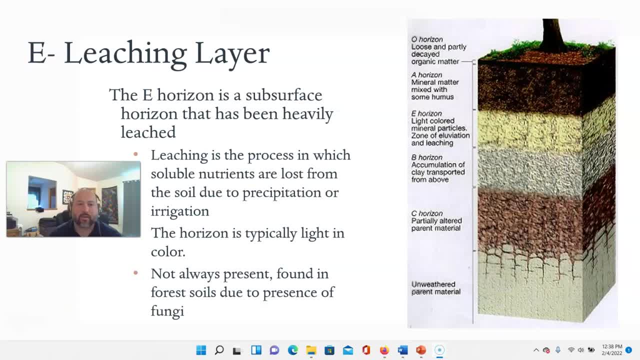 So move myself out of the way so you can see the picture clearly. So if it's a forest horizon, more than likely It's not totally common. It doesn't have to be there everywhere, but it's more common in a forest soil than it is in a grassland soil, where we get this E horizon right here, which is a light colored, which is a light colored zone where there's been a bunch of 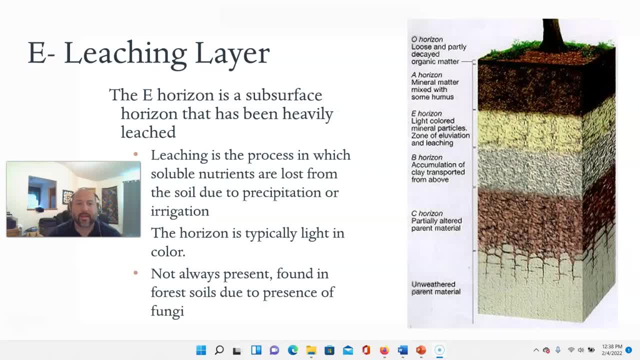 eluviation and leaching happening and it's E for eluviation, which leaching and eluviation really mean the same thing. One of the big things that's important to understand about an E horizon- if it's there- is that the reason it's got that light color to it is because the dark, the organic matter and the minerals, that stuff on the top soil has worked its way down, but it has leached through that layer. 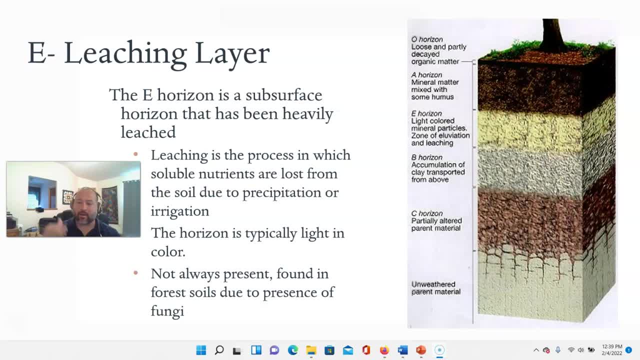 So the next layer below is actually going to be a little bit darker than this one, because all that's going to be left in this E horizon are all the minerals that didn't get leached, And so those are going to be of usually of a lighter color. 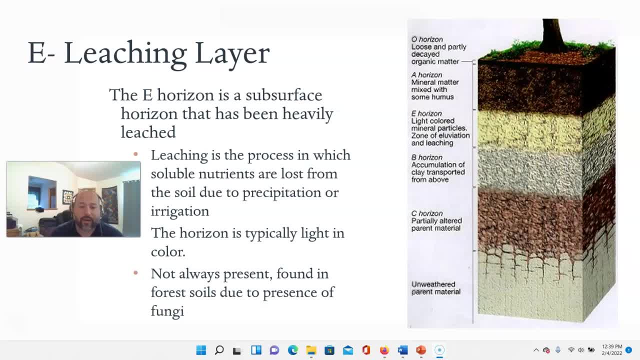 Usually an E layer, if it's found, is found in in the forest. due to the presence of fungi, in the forest, as opposed to grassland soils, are more bacteria dominated in terms of microorganisms. Just to go over it again, leaching is the process in which soluble nutrients are lost from the soil due to precipitation or irrigation. 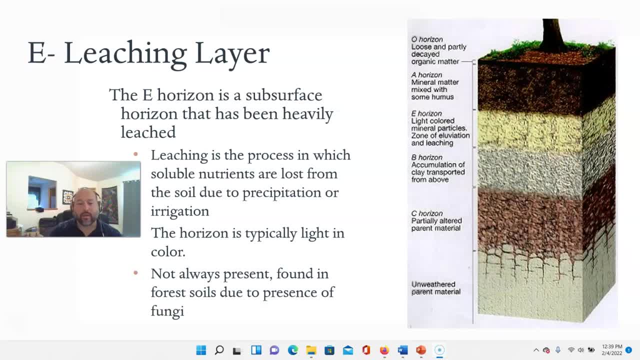 Or really, in this case, lost from one layer of the soil to the next one. Like I said before, the E layer is not seen in every single forest layer, but you could see it there And it's usually pretty distinct because it's got that light color to it. 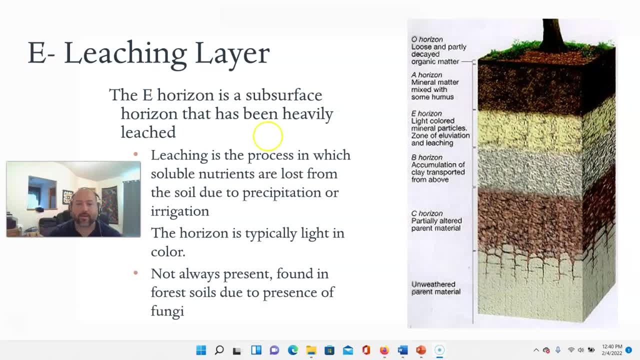 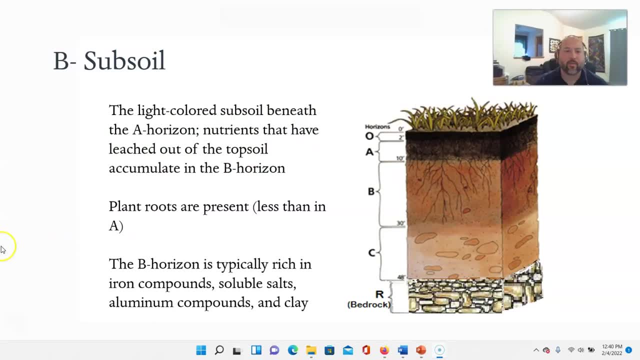 And it just goes from dark to light and then back to a darker color again. All right, put myself back up here and out of the way So. So then that takes us to the subsoil. So, looking at this diagram on the right: 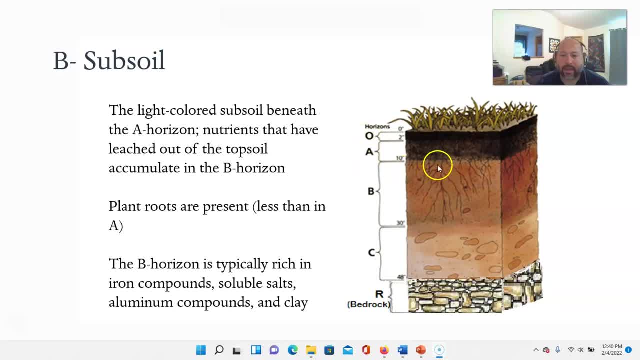 So if this was a forest soil, we would have gone O A, E, B, C, R, But we're looking at a grassland soil, So it's just O A, B, C, R. So now we're at B right here, which is the subsoil. 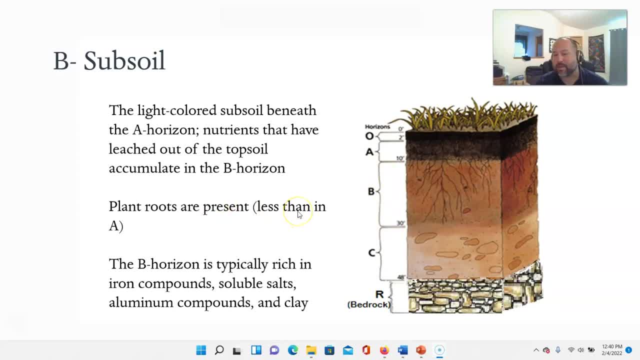 So you can see, we'll still get some plant roots present, but much less than we're in our A layer or our topsoil layer, And we're going to get a lighter colored soil because, Because we, the nutrients have leached out of the topsoil. 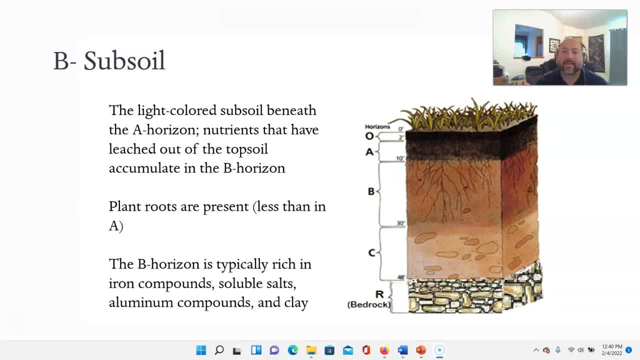 They have accumulated in the B horizon, but not there's definitely not as many, And then there's definitely not that high presence of organic matter which really gives us that much darker color. The B horizon is typically rich in iron compounds, soluble salts, aluminum compounds and clay. 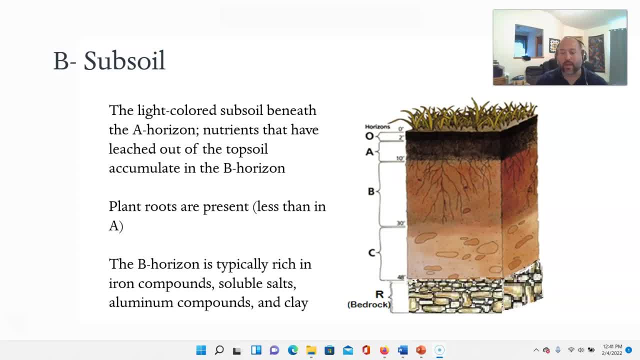 And those. because of those, the presence of those minerals and those compounds In the soil, you're going to get a much lighter color as well, And especially with the iron compounds, because they're easily oxidized- easily oxidized- that you're going to get a lighter color, kind of a rust color in some places. 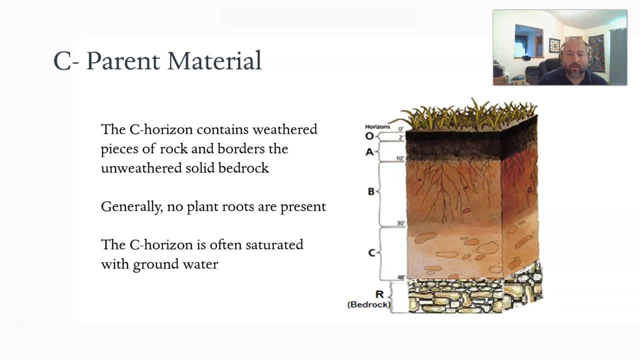 Our next layer down is our parent material. so our parent material is the sea horizon. Sometimes they'll just say like weathered bedrock And all we're saying is That the sea horizon used to be the horizon which all the soil used to be down there in the horizon. 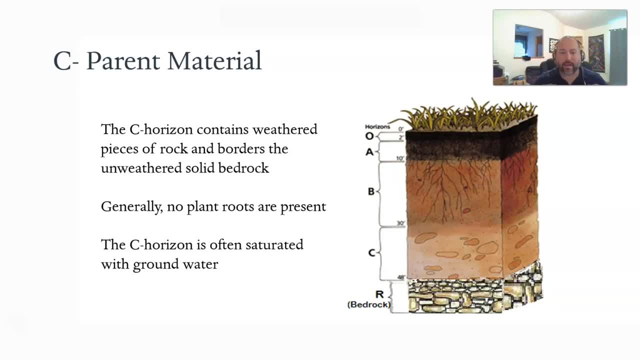 But instead of the, this consolidated rock, the unweathered solid bedrock in the sea layer. we have weathered bedrock, So it's been through water or wind, erosion or water and air processes. The rocks as broken up into different pieces- and those different pieces then are- are just sitting there. 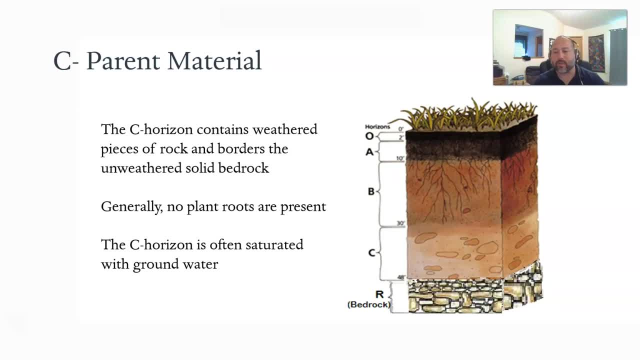 And then what's? What's interesting about that is we usually don't get plant roots going that deep, but then that's now where our groundwater storage usually will happen. The sea horizon is often the one that's going to be saturated with groundwater. 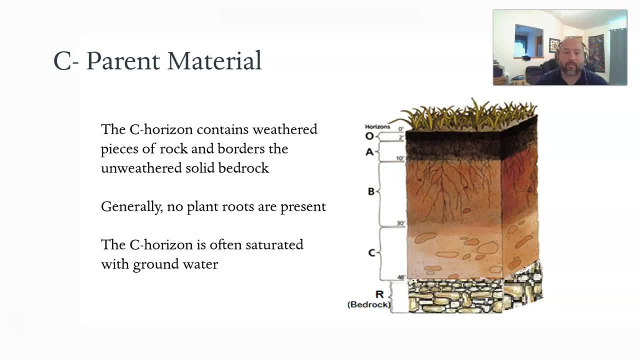 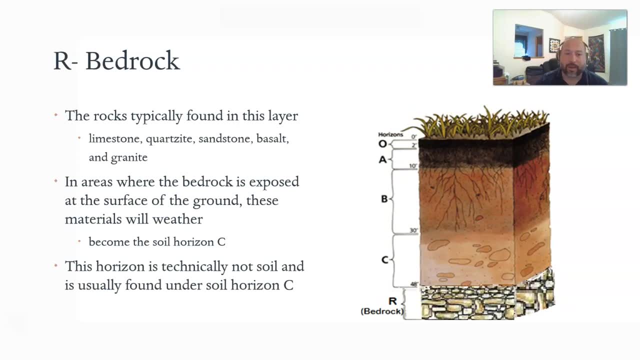 If you have an underground aquifer below you, that's where it's going to form, And then that takes us to the last layer, which is the bedrock, the rocks that are typically found in bedrock, things like limestone, quartzite. 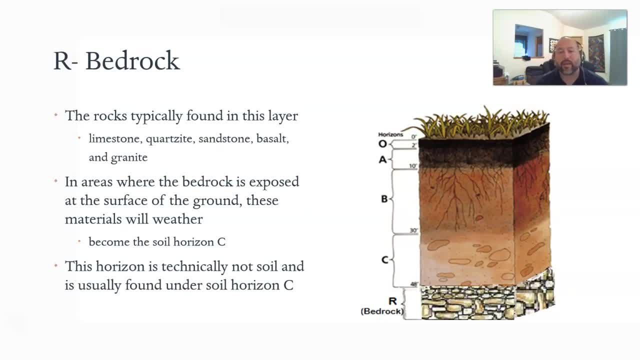 sandstone, basalt, granite granite is the one in the sierra nevadas down here. that's, that's, uh, usually our parent material for the for the southern sierra nevadas. so that's that's the bedrock for that area and we know that because there's big pieces of it sticking out of the. 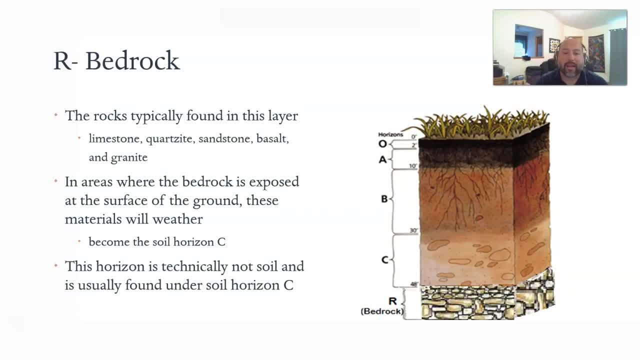 ground, like el capitan. in areas where the bedrock is exposed at the surface of the ground, these materials will weather. so the el capitan half dome, those big pieces of granite sticking out in yosemite, don't won't look exactly the same as the granite that's under the ground. because, um because, 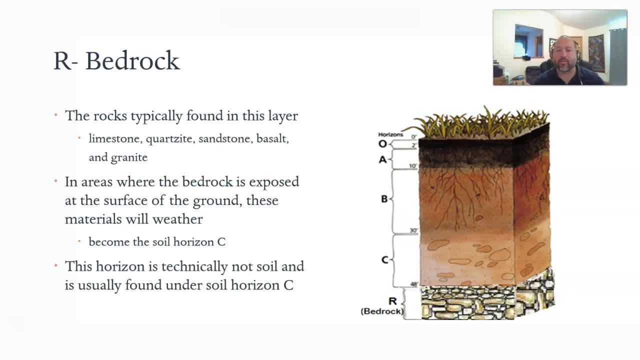 that the, the unweathered bedrock hasn't gone through that weathering process. if the bedrock gets exposed, it should weather away and and eventually years and years and years kind of become like a sea horizon where we could start to build soil. uh, that sort of thing. why won't, why won't that process happen? 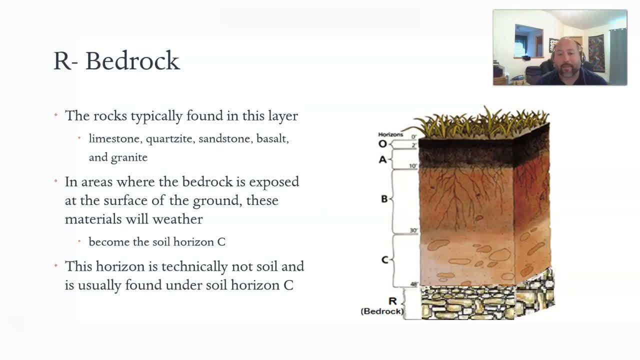 at half dome or el capitan. it could happen, but, um, they're the way that they're exposed to weather, to wind and water erosion. it's not likely that you're going to have to get enough time for soil to build up with that constant, um constant uh, wind and water. 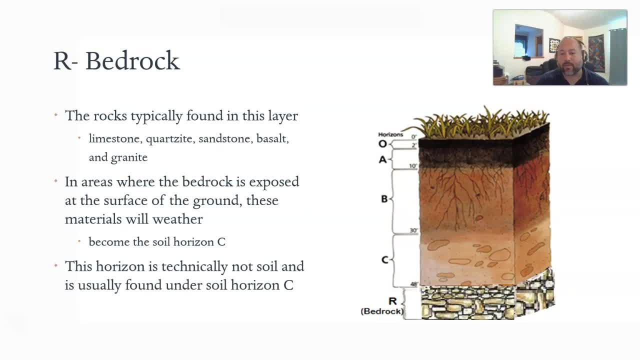 erosion happening. uh, some some people don't look at this as a as a horizon. um, because it's not technically soil, it's everything before soil, but it is our foundation that our soil builds upon, so it's important to know also one way to to think about. we just talked about the sea layer and why. 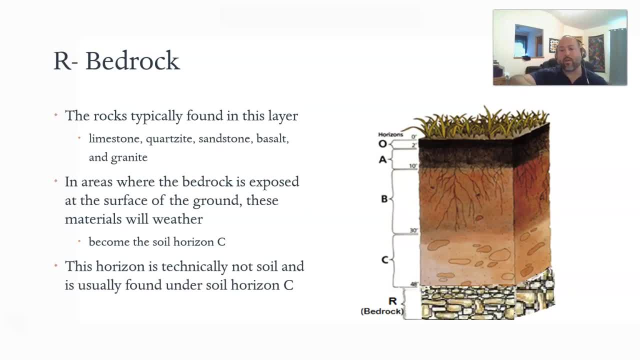 does the sea layer have groundwater in it, because all the soil we know has pores where water and air move through, but eventually it'llない浪水 시작átema hayto. yet another wave and become have new water, Pressing water and air go through time and then eventually it'. 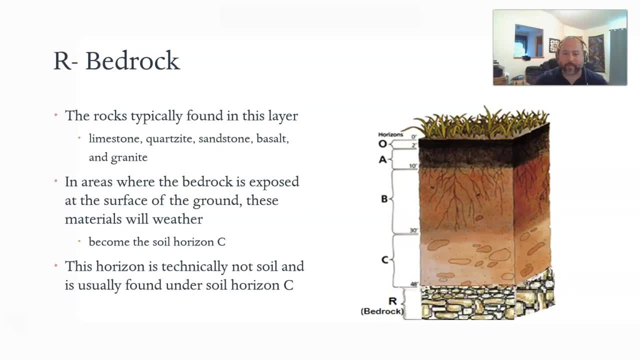 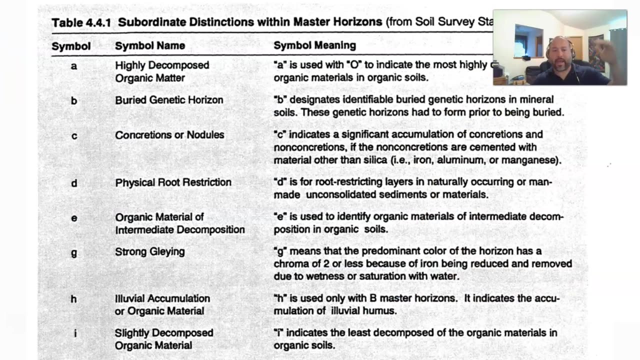 hit the unweathered bedrock, it'll hit the bottom, where now there's nowhere for it to go. so now it puddles up and pulls up, and that's how we could start to build a groundwater supply. so those were our master horizons: o-a-e-b-c-r. those are our master horizons. the organic layer. 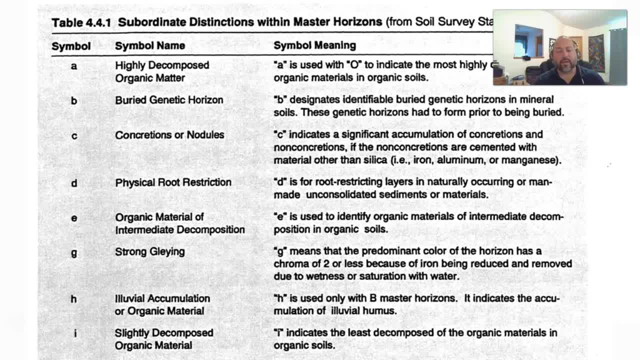 the topsoil, the uh alleviation layer, or the leaching layer, the subsoil, the parent material layer, and then the bedrock. and then we also have these uh, these lowercase letter distinctions, which are trying to tell us something specific about our, our master horizon. and so an example. so if 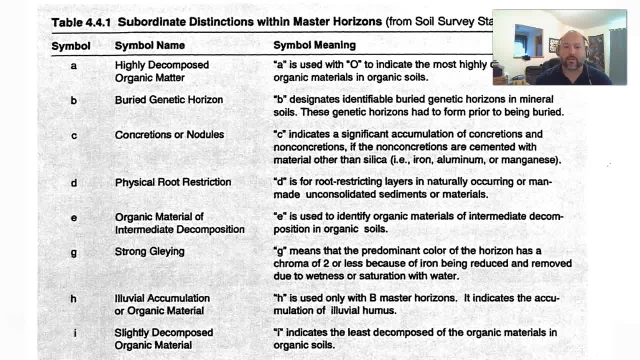 we see something where the lowercase a is used and it's usually it tells you right here it's used with the o to indicate the most highly decomposed organic materials in organic soils. or if we look at something that you'll see come up sometimes and probably not great, depending on what you're. 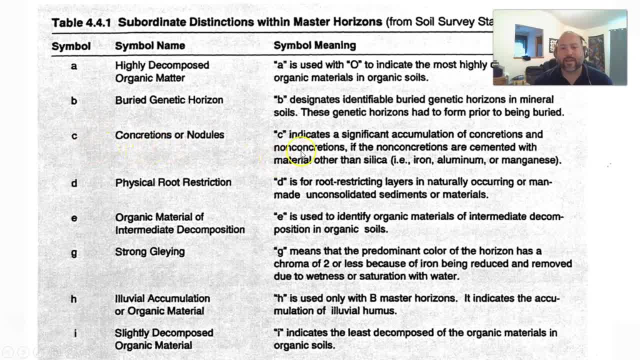 trying to do with the soil? is c for concretions? it says c indicates a significant accumulation of concretions and non-concretions. if the non-concretions are cemented with material other than silica, iron, aluminum or manganese, d would also be another one that you'd. 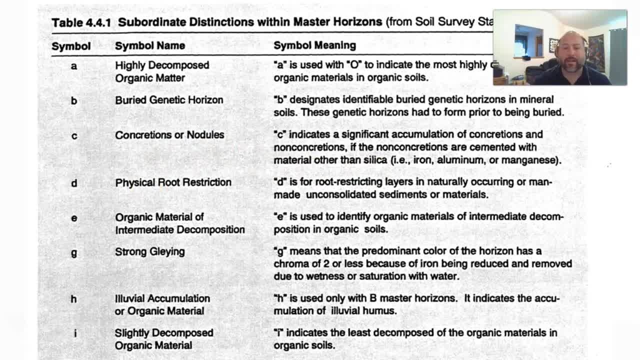 want to look at if you're looking for a material that's not cemented with material other than silica, iron, aluminum or manganese. d would also be another one that you'd want to know about, but you wouldn't be too happy about it. d is for physical root restriction, so it's for root restricting. 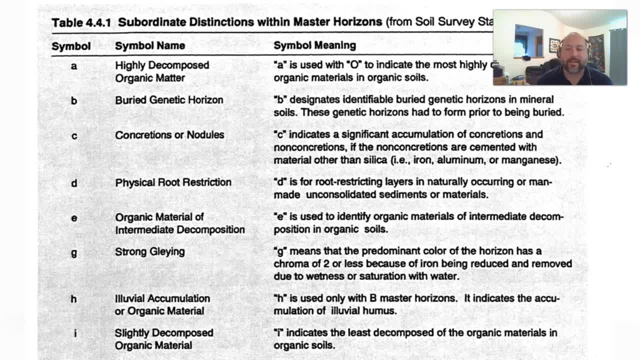 layers and naturally occurring or man-made unconsolidated sediments or materials. g. strong g means that the predominant color of the horizon has a chroma of two or less. because of iron being reduced and removed due to wetness or saturation with the water. you can see these kind of go on you. 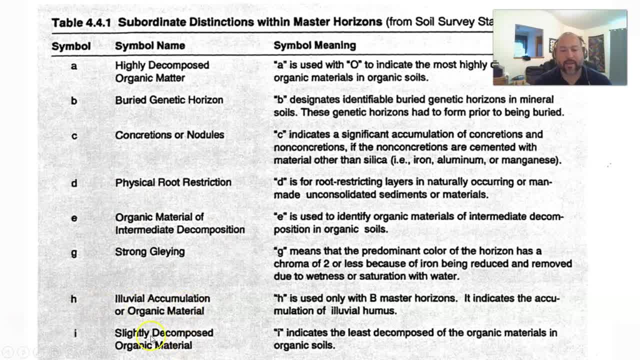 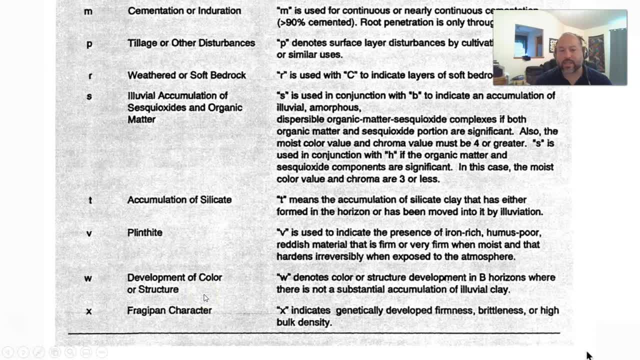 know: h for elute alluvial accumulation, i for slightly decomposed organic material. there's, there's more than this. this is just kind of some examples that i got for you. r for weathered or soft bedrock, so r is used with c lit to indicate layers of soft bedrock. so you would 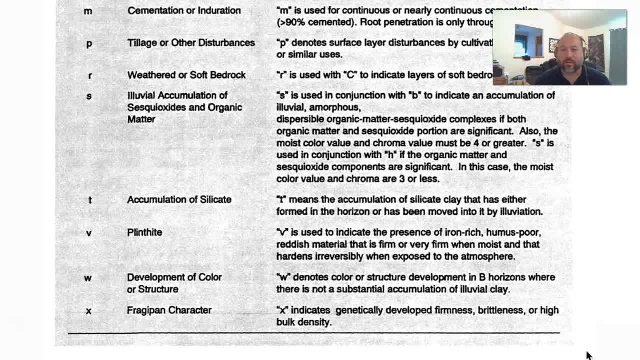 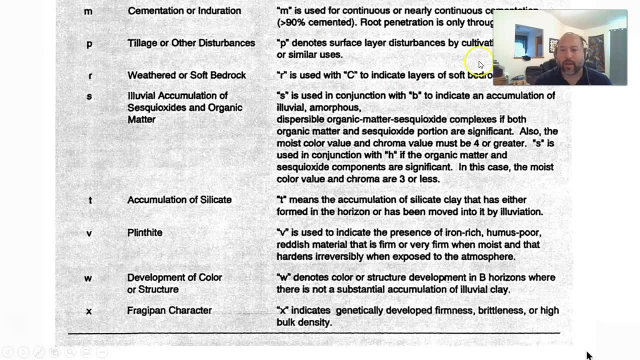 see r being used with c. you wouldn't really see it used the, the lowercase r, with any layers other than c. uh, we talked about p before because i said you could have an ap layer, which is a top soil that's been plowed, or some other disturbance by cultivation or pasturing. pasturing m for. 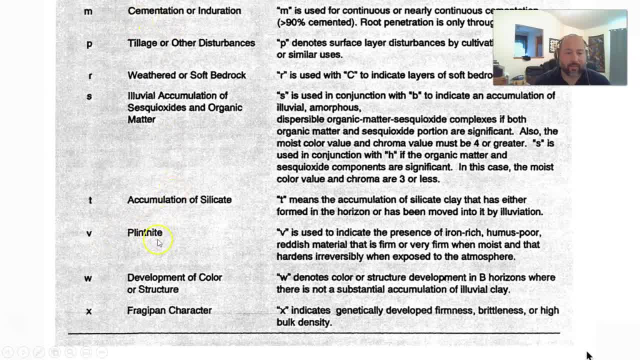 cementation. uh, you got v, would be plentite. so v is used to indicate the presence of iron, which iron rich, humus, poor, reddish material that is firm or very firm when moist and that hardens irreversibly when it hardens irreversibly when it hardens. it hardens irreversibly when it hardens. 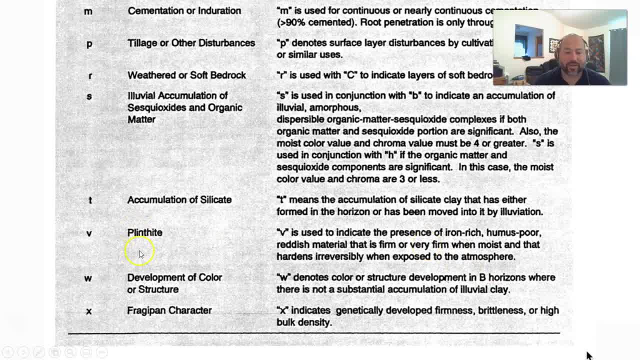 when it hardens irreversibly, when it hardens irreversibly, when it hardens irreversibly when it exposed to the atmosphere. so that's, that's an interesting one. x for frangipane, character x indicates genetically developed firmness, brittleness or high bulk density. so there's. 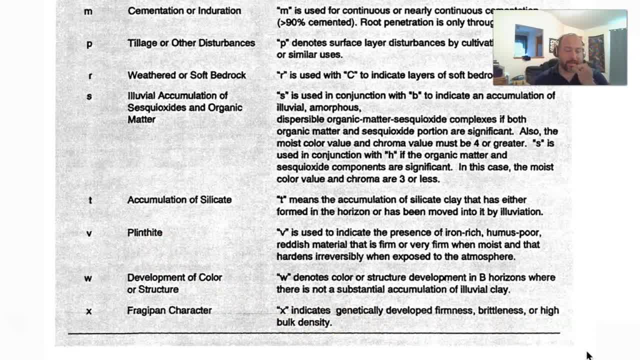 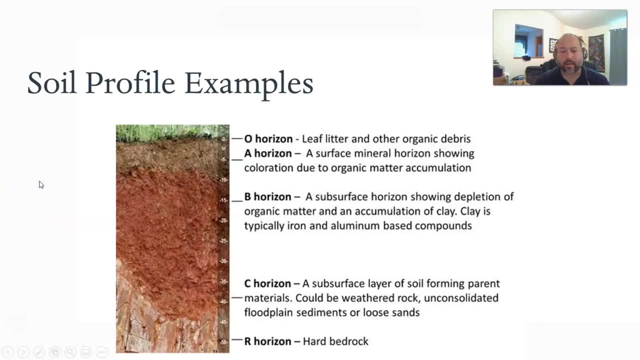 a few examples of what the you know, the specific, the specific characterization that the lowercase letter is trying to make of that master horizon. so let's take a look. so here's kind of our basic grassland soil, our o, a, b, c, r layers and where they 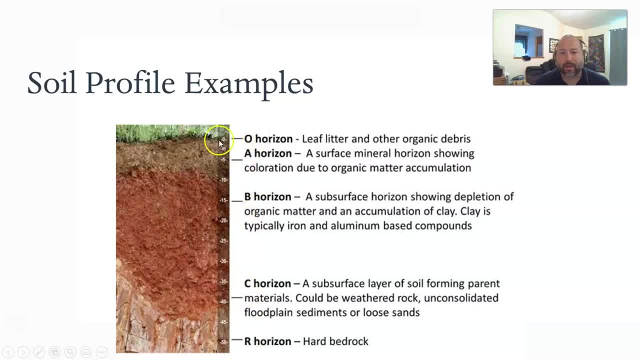 start. so this is in inches. so right up here at the top we've got our o layer and we've got our o layer. and then we go down and we have our a layer here so we can see a little change in color. so you can see, right here at the top you've got your o layer, real dark color there. we get to our 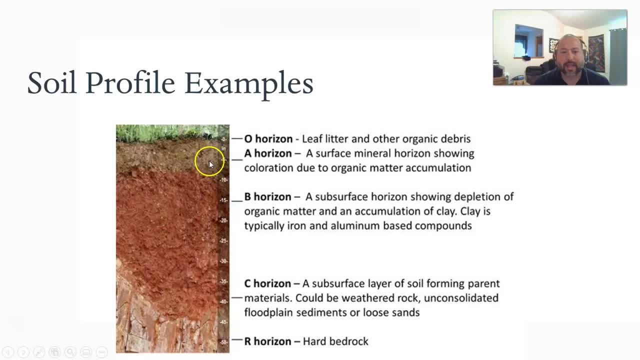 a layer where we have our o layer, and then we go down and we have our a layer here, so we can see also have a darker color, but not as, not anywhere near as dark as that o layer at the top. we then get down to our b layer, our subsoil, and you can see that this- uh, we've got the depletion of organic. 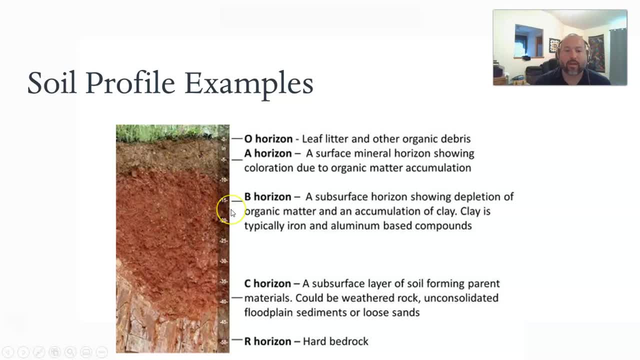 matter, because we don't have that, that brown or that dark, our dark brown color that we see up above. but we also see an accumulation of clay, and clay is typically iron and aluminum based compounds in it, and we can see that that is more than likely true because of this. 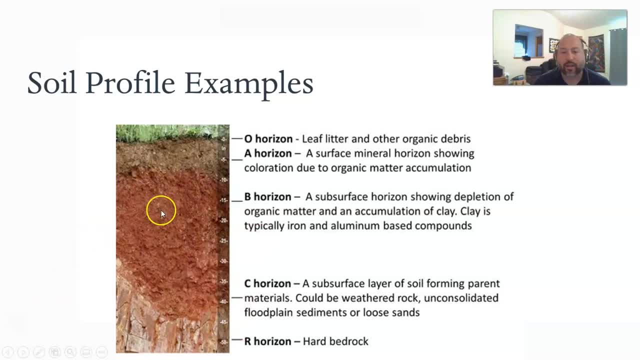 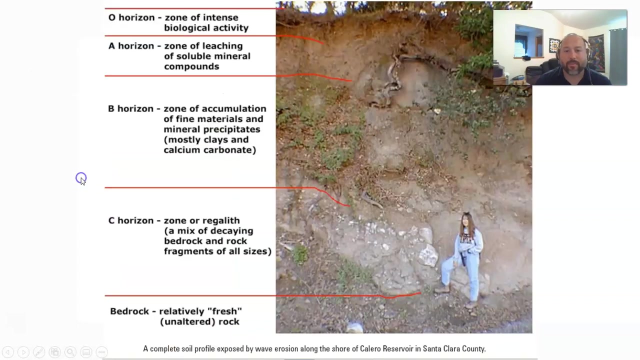 bright reddish orange color that we see in our b layer. we then see our c layer down here, where we see, uh, our, our parent material or our weathered rock material, and then you can see down here where we actually hit the hard bedrock and the the un, the unweathered bedrock. another look at it. so 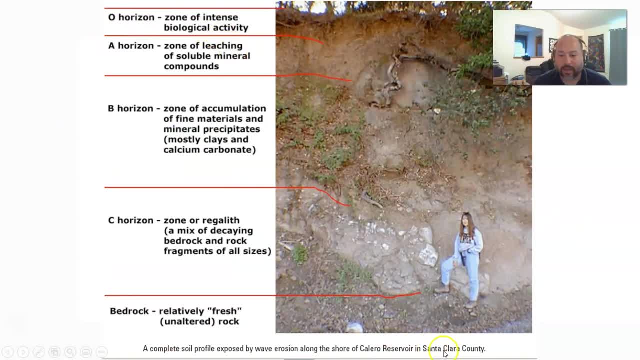 in this soil profile here which is up in santa clara county. so we've got our o horizon up top, way up top here. we then have our a horizon. we've got a b horizon, a subsoil. we got our c horizon, which is: this is a really good look at a c horizon to me. 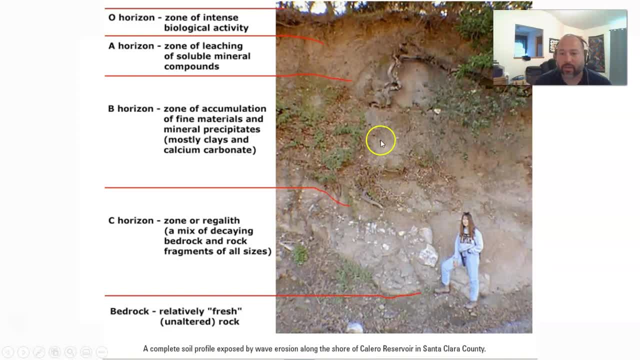 because you can see that there's still the soil and all the soil development up above. but then you can also see the big pieces of of weathered, um, of weathered bedrock, and you know how it. you can see the big pieces of weathered, uh, of weathered bedrock, and you know how it. 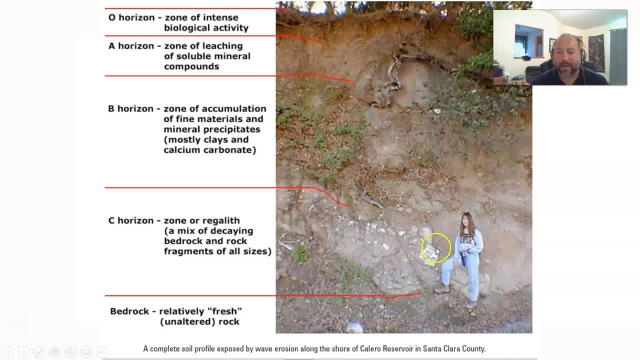 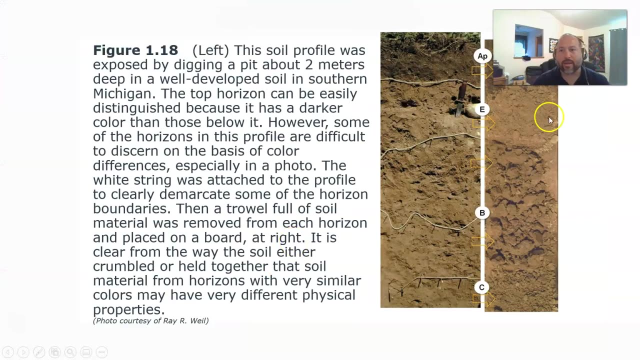 used to be the you know part of the bedrock, but now it is weathered into much smaller pieces and then we've got our bedrock feature down below. let me go back one. there we go, so here's another. look, i'm gonna kind of move myself. do my best to get myself. 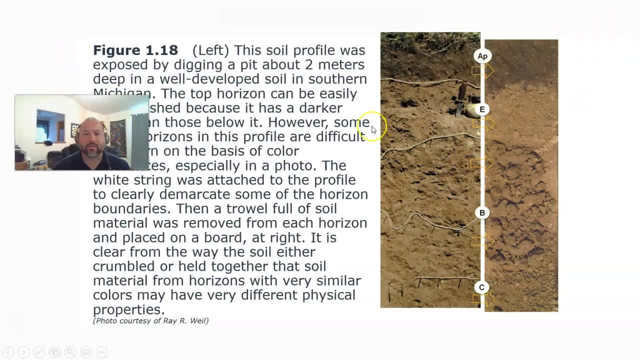 out of the way here, just so you can see the pictures. so right here we start off with an ap layer, so that's top soil that's been plowed or cultivated or changed in some way like that. we then go to an e layer where we that's, that's that leaching layer that we have here. so if we 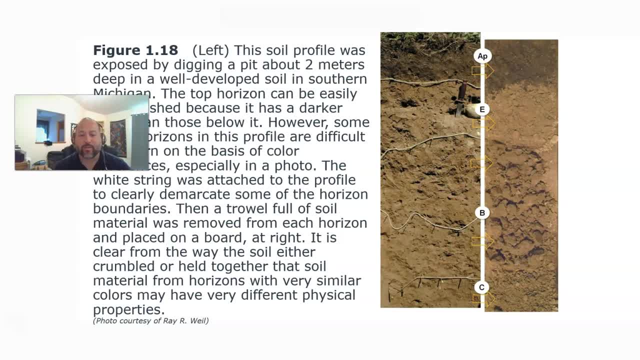 didn't know anything about it. we probably assume that the soil might be forested with with trees or shrubs up above, just because that's that's much more common, um to think so. we can see that our e layer it's a little bit lighter in color and then when we go down below we can see it actually darkens. 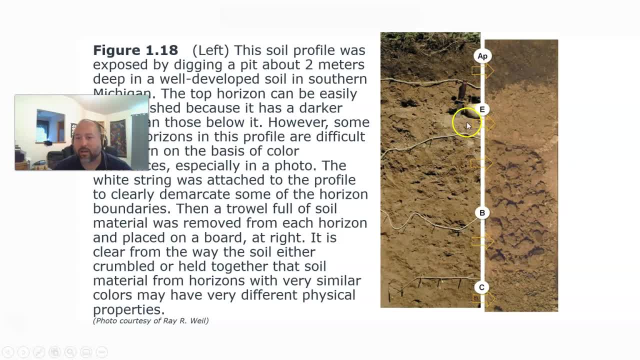 back up again as compared to the lighter color here in this e layer. we then have a b layer for our subsoil and a c layer where we get to our um, our weathered, our weathered bedrock. i'll move myself out of the way now if you want to. 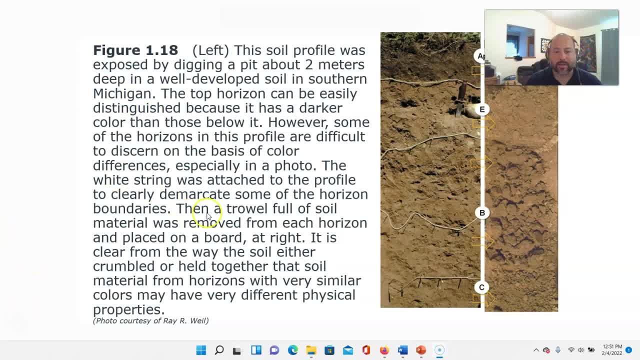 to you read, or you know, you can pause and read- how they uh describe this uh soil from from southern michigan, and it's um, it's just the big thing with morphology and the big thing with what we're doing, uh, today is really trying to get you to just um, see these differences and just to start to be. 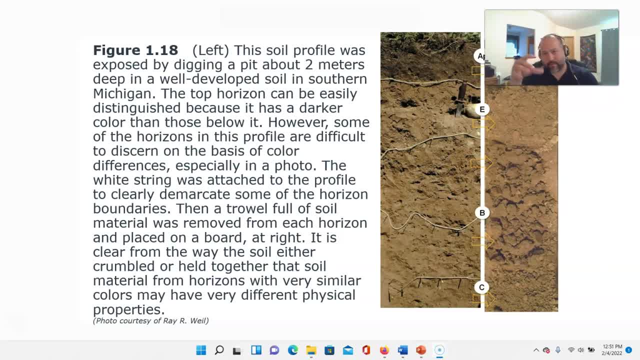 able to look at soil and say: well, wait, that looks different from that. and how are we going to classify that? and how are we going to say that this is different from that? because it obviously with our eyes, we can see it and we can see that difference. but 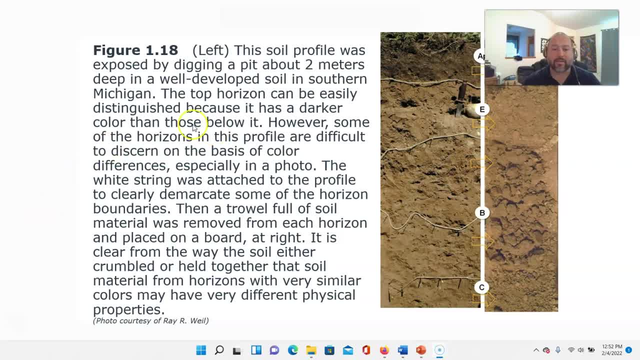 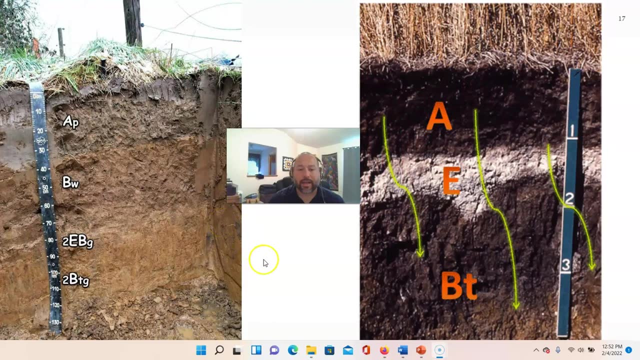 how do we actually express it or how do we make it so that everybody else who sees the same distinction can can understand it and classify it in the same way. here i'll move myself to the middle here and so kind of looking at the same thing here. 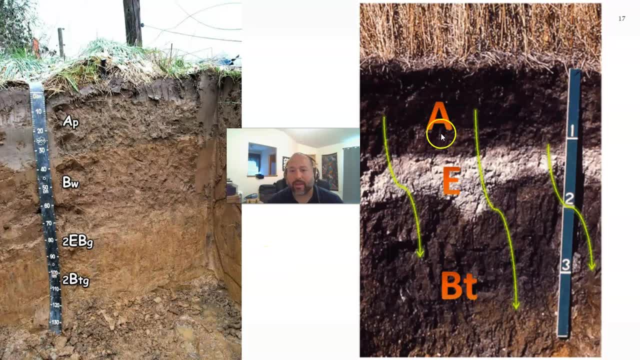 you know a couple different uh ways to look at. so here we've got um, here's our, our surface, and then our our surface litter at the top. we've got our a layer here, our top soil, a nice dark top soil. we definitely have a really obvious e layer here. uh, an alleviation, a leaching layer. 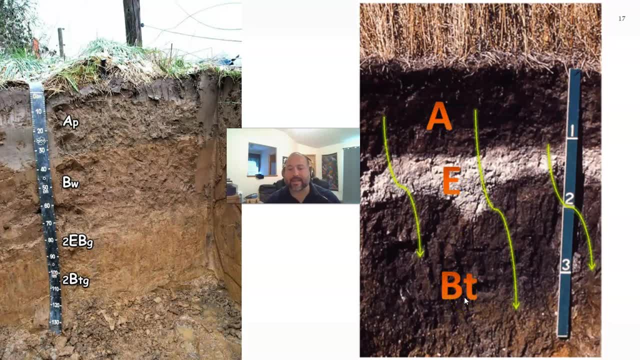 here, and then we've got a b layer and it's a bt layer. so then we see that strong, that strong leaching layer that leads to this bt. uh t is the idea of uh, of an accumulation of silicate clays. so that's what the, that's what that t stands for there on the right, on the left. 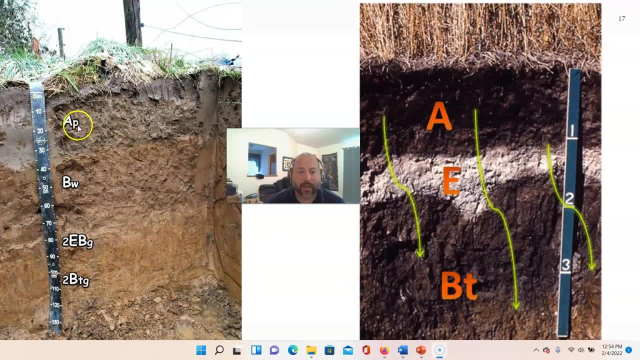 here you see another one of these ap layers. so that's our top soil that's been plowed or or cultivated in some way. we see a bw and w stands for a change, a change in in the b layer due to, or some sort of, a change in color or structure. we see here that this one. so it says: 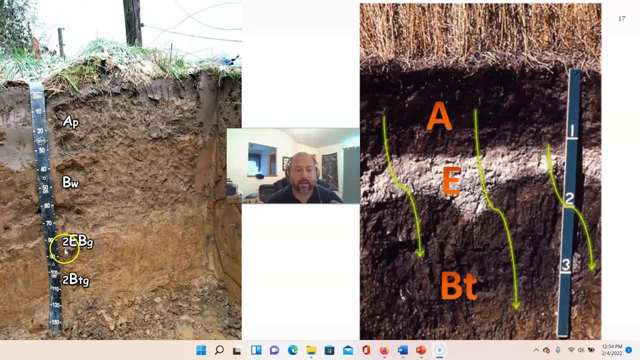 uh, two: e, b, g, so the two here. we talked about that at the beginning. it's not totally common, but it does happen where it means that there were two different parent materials. so there was something, some process that happened and then some other process that happened. so there's, there's. 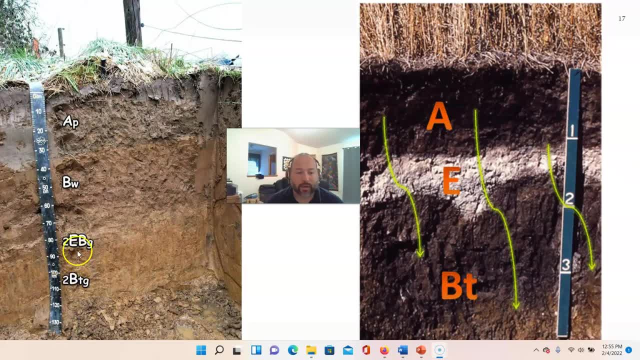 two different parent materials, um, within this soil, and then this is an e, an e and a b layer combined with a- b, and then there's a b layer down below and then the g. the lower is g, that means um glaying, and then we can see the t again here. so that's that accumulation of 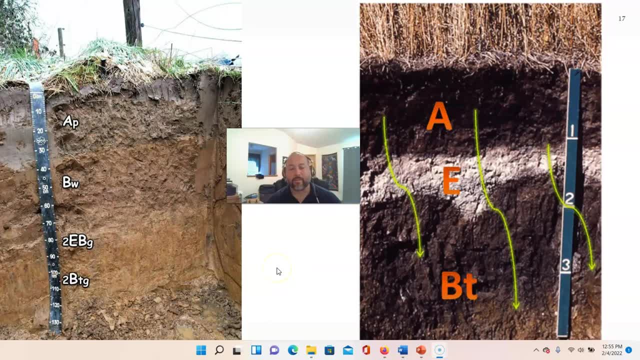 silicate clays and the glaying as well, and i'm not going to, you know, pretend that you're going to memorize all these things and and you know, it's all going to come to you right away, but there's lots of glossaries and lots of field manuals and things that'll have a list of this. 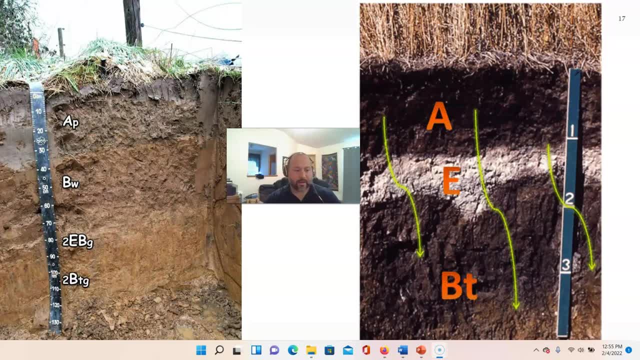 and once you figure it out and you know what you're kind of looking at, then you can just look it up and say: oh okay, it's, you know there's a, there's a g here- i know i can look on the list- g. g means glaying. what's glaying again? oh yeah, this is what it means and that's kind of the. 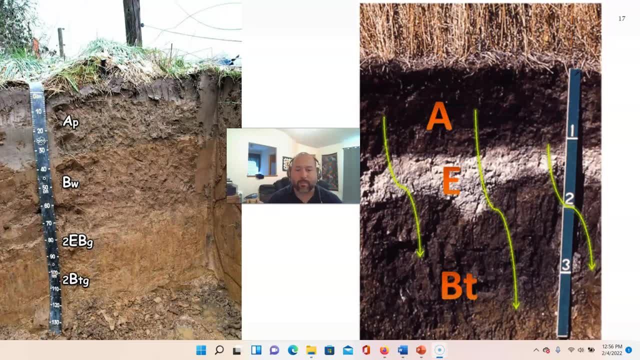 process. but as long as we have a lot of these descriptors in place and we can use them and we start making what our eyes see match up to what the description is, that's when we're you know, we're off and running and everything's golden in terms of of really trying to get a good description. 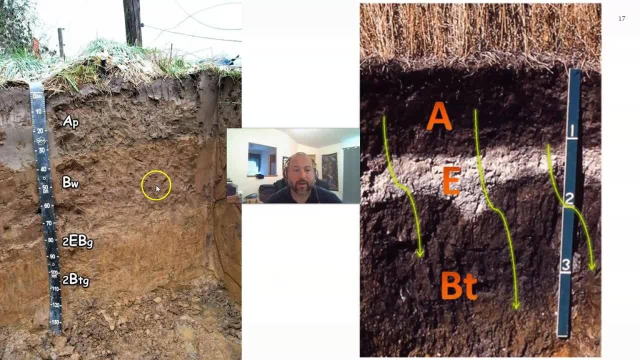 of a soil profile here, so just kind of going over some of the stuff from before. right soil, uh, pedon, if we, you know, cut a perfect hexagonal shape out of that, but we're looking at one face of that pedon. so this whole thing is a profile. then we've got our horizons within the profile of our different. 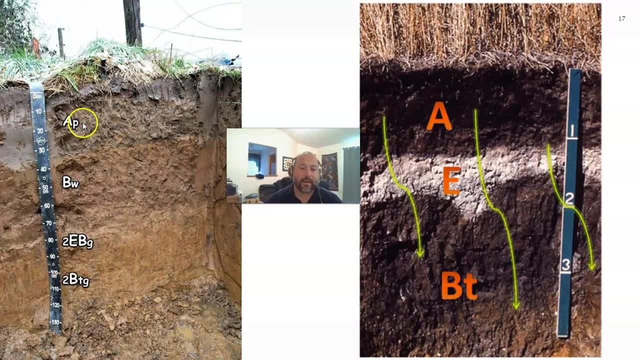 layers within that profile. and then we've got master horizons. these capital letters here, a, b, e, b and b- here are lowercase letters which are specific um, specific um designations or specific characteristics about that master horizon. if we have a number before the master horizon, that means that it's 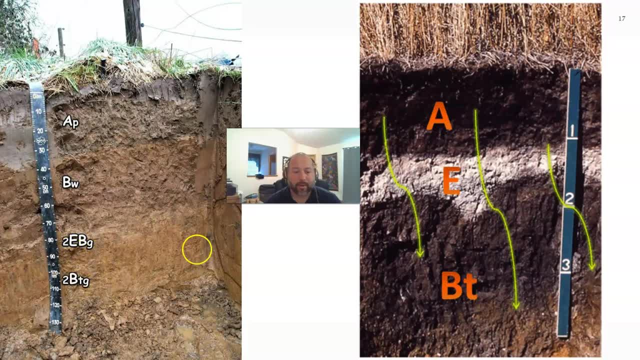 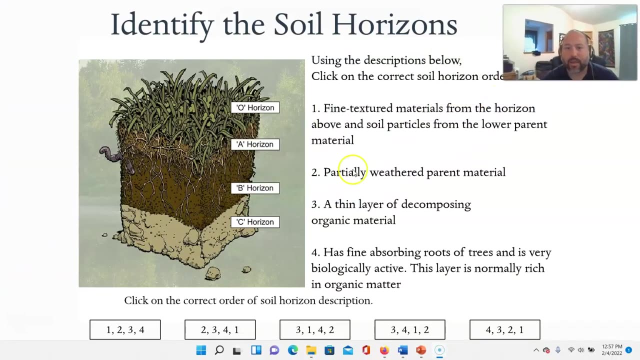 uh, there's more than one parent material. and then if we add a number after um, the lowercase letter, then there's subdivisions: um, within the uh, within the horizon. so we're going to go and get that top right and then we're going to go ahead and we're going to go. 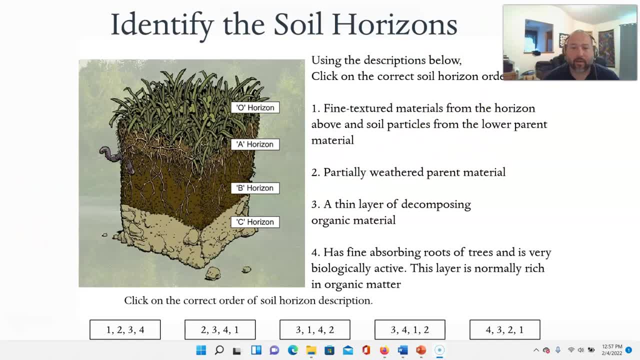 down and we're going to go and add a little bit more and we're going to add it up and we're going to go back up here to the top, right out of the way. and so just a little kind of quick quiz right here on our, on our basic layers of a grassland soil: soil, our o horizon, our a horizon, our b horizon. 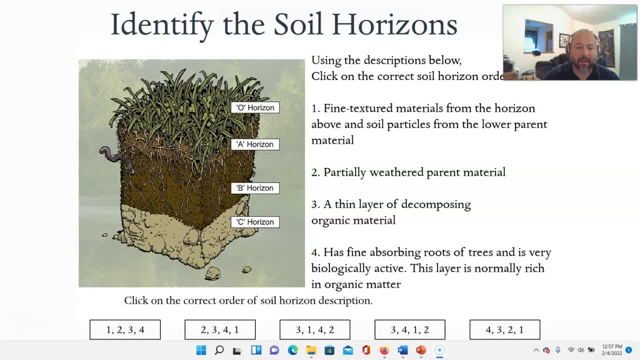 our c horizon. so go ahead and, um, look at this. read the descriptions that i have there in one, two, three that i put down there. which order is the correct if we're going to describe top to bottom the o layer, a layer, b layer and c layer? so go ahead and pause the video. all right, so did you guess? 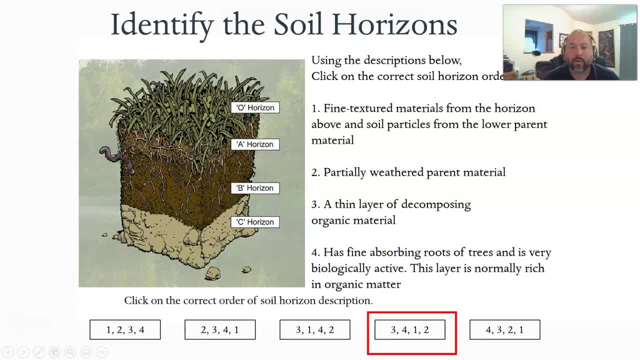 that one three, four, one, two. so if we're describing the o layer, a thin layer of decomposing organic material, our a layer has fine absorbing roots of trees and is very biologically active, and that this layer is normally rich in organic matter. our b layer then has fine textured materials from the 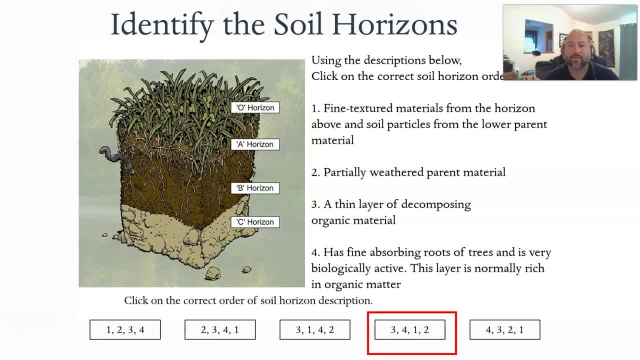 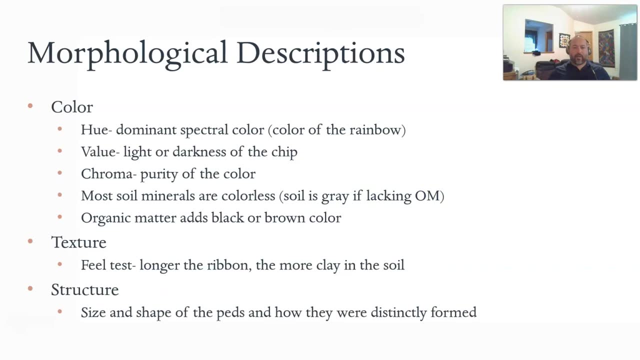 horizon above the things that reach down and soil particles from the lower parent material right, the b horizon sitting right above that parent material, and then, number two, partially weathered parent material. that's the description of our c horizon. you so other ways that we're going to describe the soil or focus on describing a soil profile? 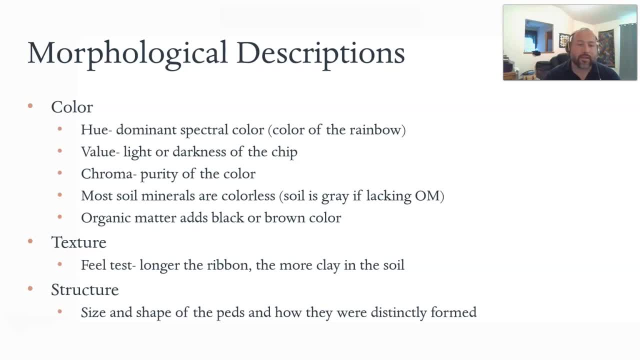 we focus on the color, so using the munsell color charts, that's um, that's the most common way of doing it. they focus on three values, which are the hue, the value and the chroma. the hue is your dominant spectral color or your color of the rainbow, the ones that we focus on using in class. 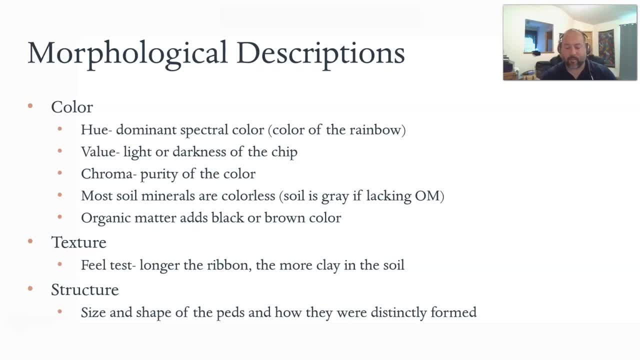 the. they'll say why we r after them. and y? r stands for yellow, red, and that's how we get our um, our brownish, our brownish colors that we, that we see a lot in soils, is some sort of combination of yellow and red and or. 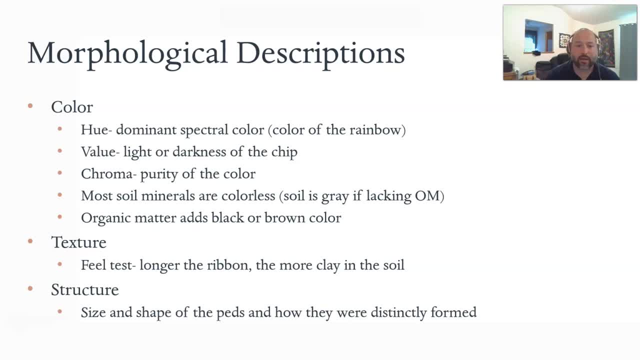 somewhere in between. so that's our dominant spectral color. our value is going to be the lightness or darkness of the chip, or, you know, the soil that we're looking at, the lightness or darkness of it, and then the chroma is the purity of the color. so how pure is the color, or or you? 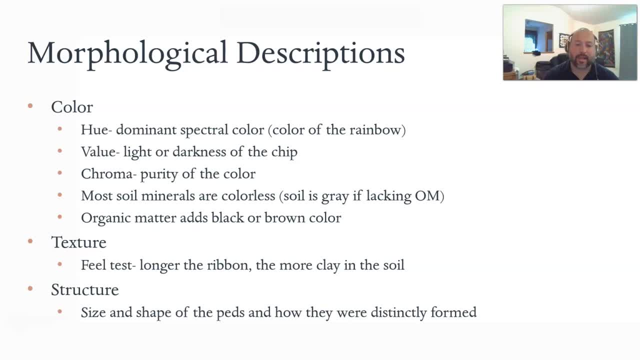 know what else is in um, in that color that makes it, you know, lighter or darker or you know not as rich, you know more dull, not as rich sort of a thing is is the way that i would look at, because if we're saying value is lightness or darkness, then chroma, i would say, is kind of the richness. 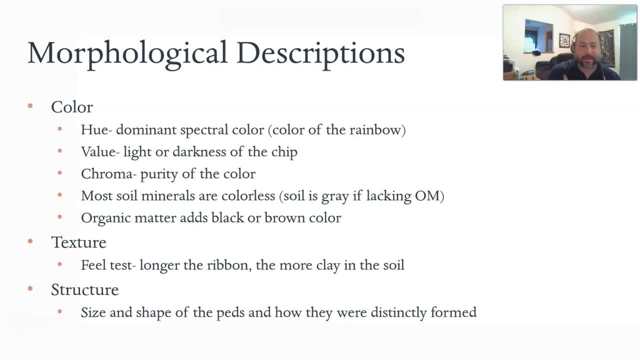 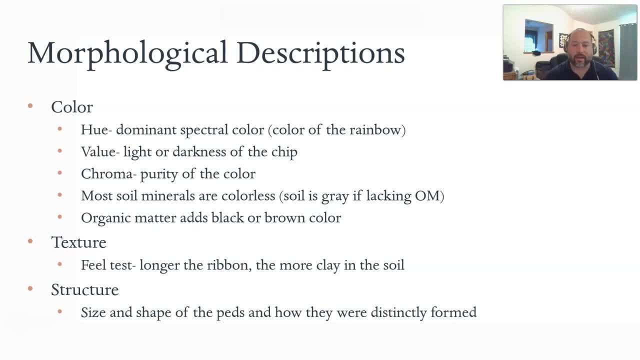 matter in it and it's going to be kind of obvious color-wise that way, If the color of the soil is black or brown or reddish color, there's something else going on, something else happening there, And that's an important distinction that we can make and that's why it's important in 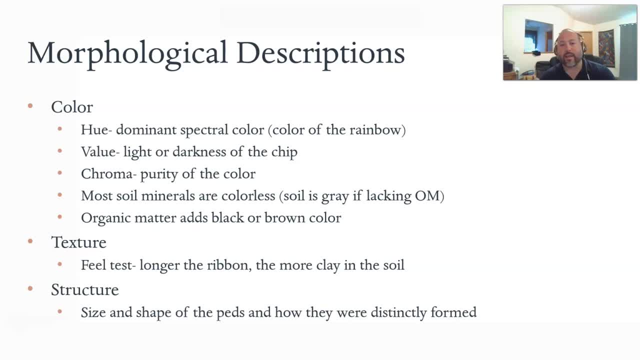 terms of a morphological description. We also can use texture. The field test is the one that we're big on, and one of the big focus points on the field test is being able to ribbon correctly between your index finger and your thumb, and the longer 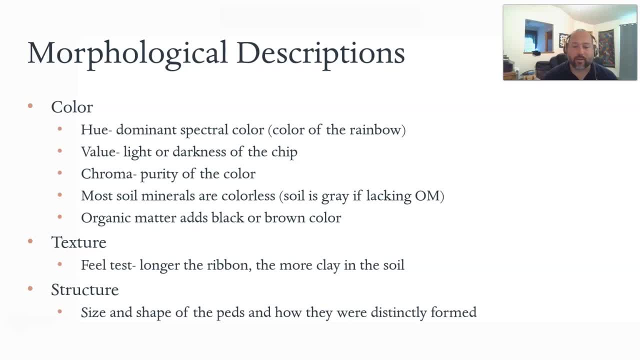 the ribbon you can make the more clay you have in your soil, And so you start to get a feel for what does sand feel like, what does clay feel like, and then silt as well, Structure the size and the shapes of the peds. 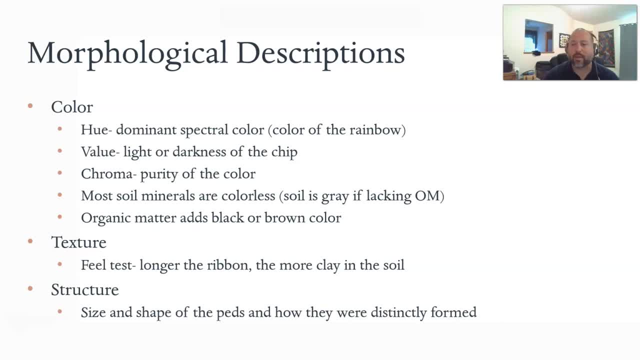 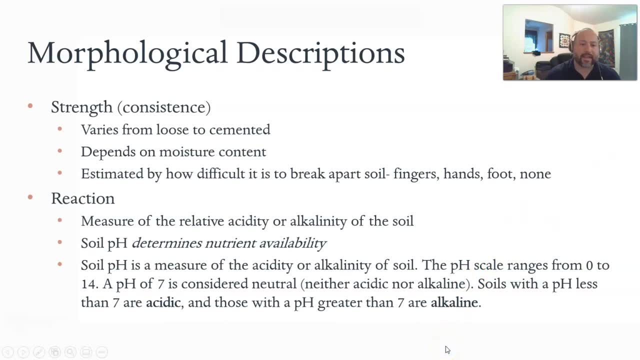 Within the soil In your soil profile and how they were distinctly formed is going to tell us a lot about the soil profile and give us a lot of good information. We're also going to look at the strength of the soil, which is also called the consistence. 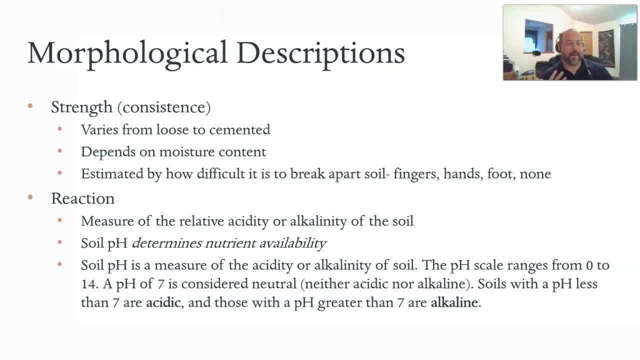 of the soil, So it can vary from loose to cemented and it's really going to depend a lot on moisture content and the way to estimate that is: just how easy is it to break the soil apart? Can you use your fingers? Do you have to use your hands together to break it apart? 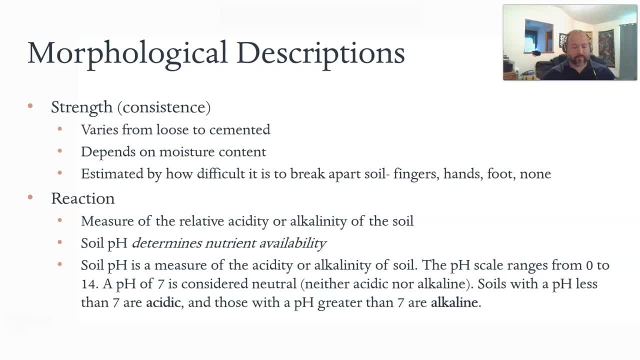 Do you have to put it up? Do you have to put it under the foot and stomp it to be able to break the soil apart, Or does it not break apart doing any of those sorts of things? We also have reaction, which is a measure of the relative acidity or alkalinity of the 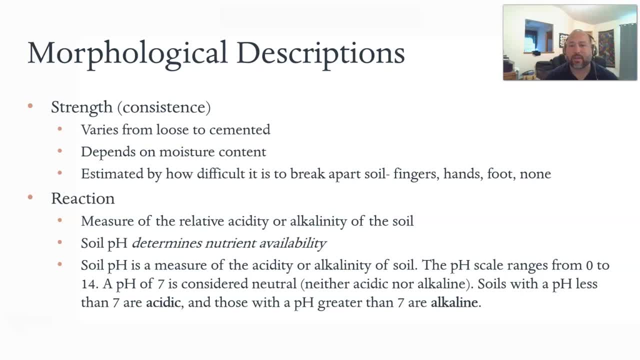 soil, which is going to be based on your soil pH, and your soil pH is going to determine your nutrient availability in the soils. So your soil pH is measured on a scale of zero to 14.. Seven is neutral, So that's where water is. 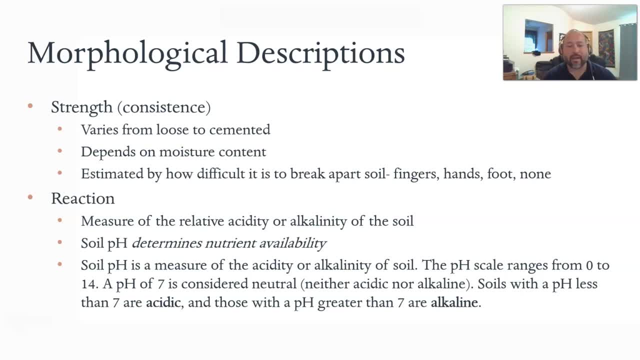 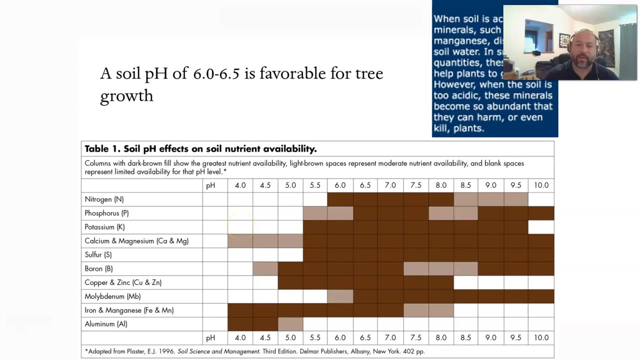 Water is neutral. It's neither acidic nor alkaline. Soils with pH of less than seven are acidic soils. Soils with pH greater than seven are alkaline soils and here's just kind of a look. Soil pH of six to six and a half is really perfect for tree growth, but you can see based. 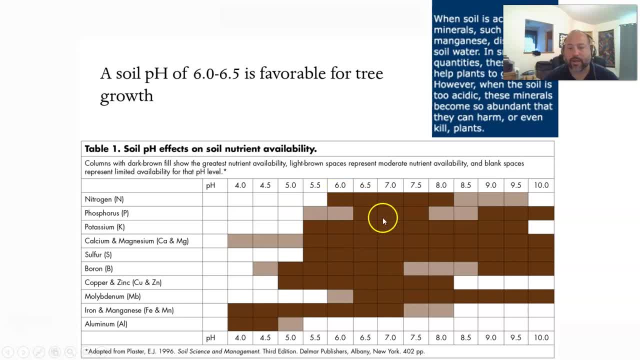 on these minerals here- and that's what's important to us- is our nutrients and how many nutrients are available and where can we get them. You can see anywhere between six and eight were probably decent, down to five and a half, maybe even were okay. 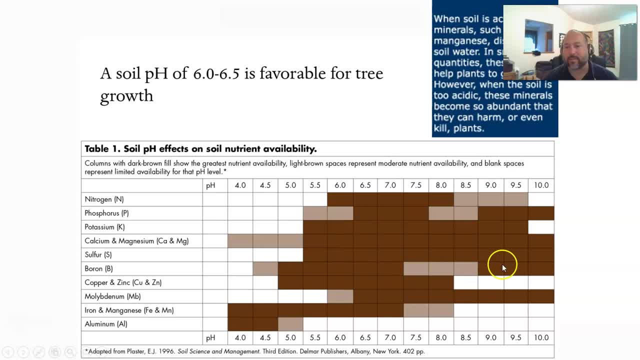 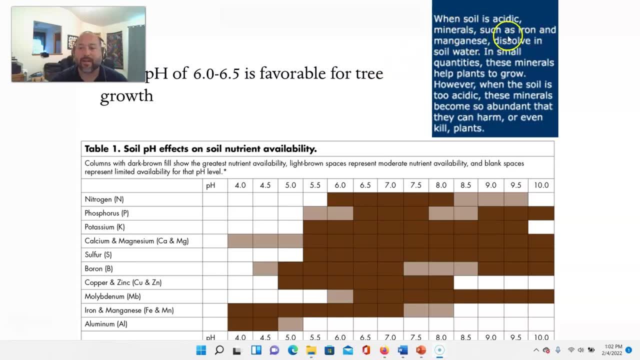 Anything there is pretty good, but anything outside of that starts to become problematic. And I'm going to slide myself over here now because I want to just talk about this little bit right here. When soil is acidic, minerals such as iron and manganese. so if we find down here here's 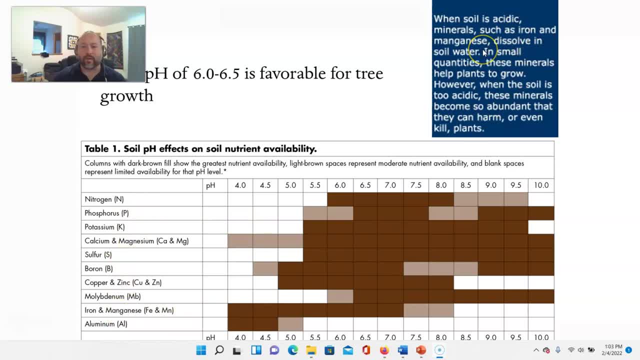 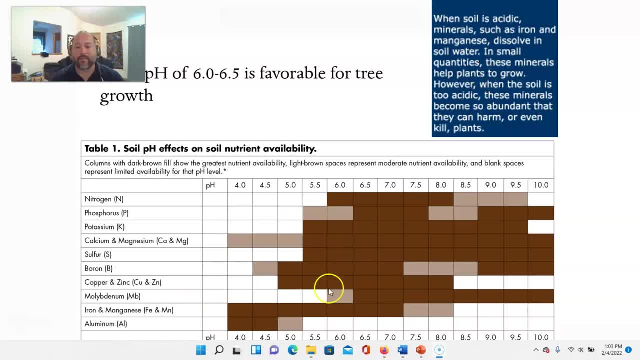 However, if your soil gets too acidic, down below four or so, then iron and manganese just start to accumulate and accumulate, and accumulate so much that they can actually harm or kill your plant, And the same thing can happen with other nutrients. So actually, in the majority of cases, some soil will decay this way or that way. right? 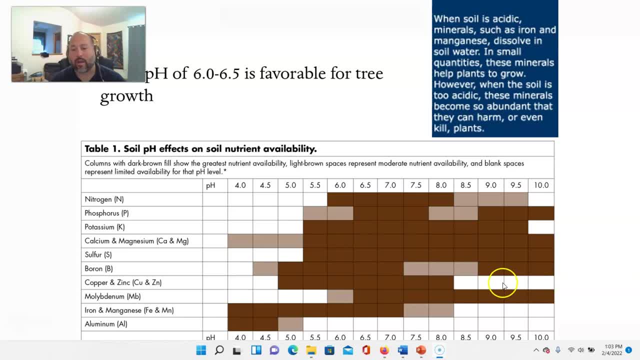 back into the reticle because they are胭 acid and they're going to be very safe and they're going to be a natural hit pick on whenuitar ester soil. This is specific to some of these different types of soil that become very excitement. 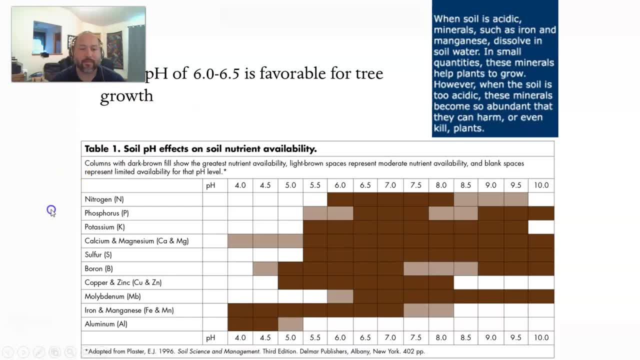 terminology for water, but we're going to get all the information that we need from that right now. We're going to try that again. Okay, Because of this, this pattern, you actually see that they're both a lot more acting then when the water is мыre��. 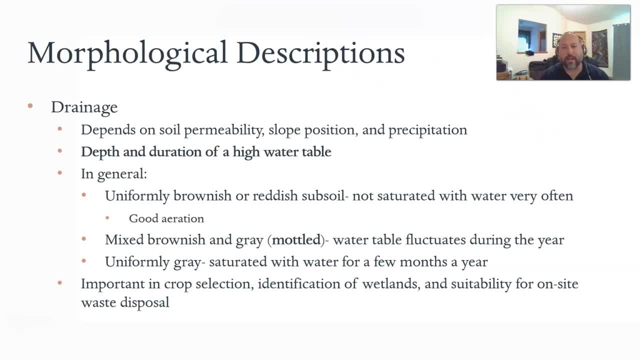 I'm on the inside, We're going to have a lot more Raisin. I just talk about Lake children, whether they're going to be green, whether they're staying alive, or now on soil permeability. so how quickly and easily does the water move through the? 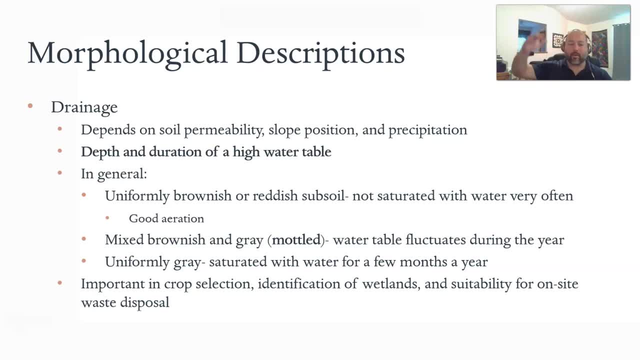 soil, the slope position, because it's going to be really important. are we? are we top of the slope, where everything's going to be expected to be? you know running downhill and you're going to get a lot of runoff issues- mid slope? are we at the bottom, like we are here in Bakersfield? we're in a valley, so we get. 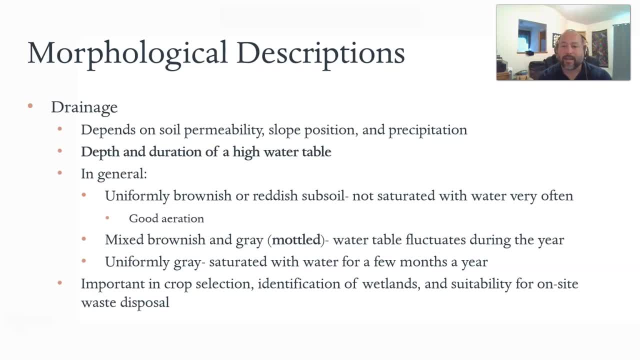 a lot of things accumulating down at us and then amount of precipitation, and so when we're talking about drainage, we're really talking about the depth and duration of a high water table, and where the water table is now. the water table is just the top of where the groundwater is in the, in the soil, and so when we're 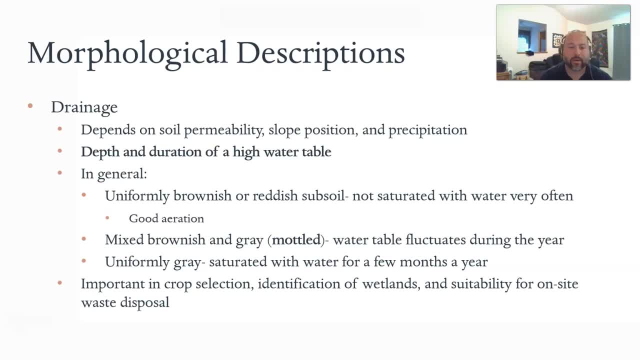 talking about drainage, we kind of got three, three basic categories. so we got uniformly brownish or reddish subsoil, so it's not saturated with water very often and you've got good aeration. you can have a mottled soil which is like a. 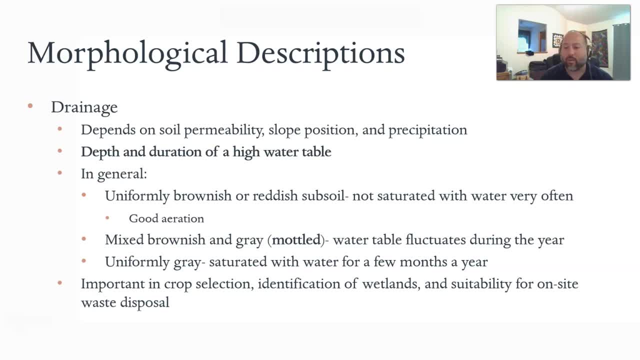 mixed brownish gray. that means that you're going to get a lot of precipitation. and you're going to get a lot of precipitation and you've got good aeration, you can have a mottled soil, which indicates that the water table will fluctuate during the year. so where you 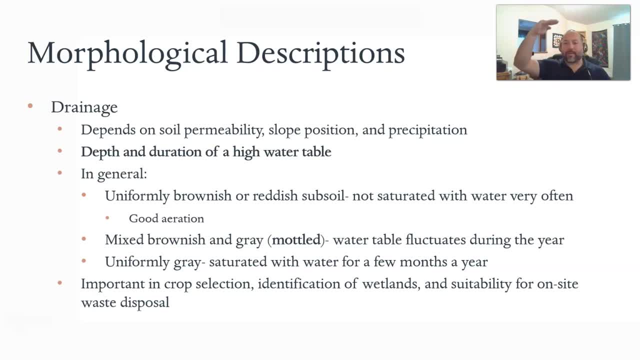 can find groundwater instead of it being here all the time. maybe sometimes it's up here, maybe sometimes the waters down here, so maybe I have to dig. you know, during the, during the winter, I don't have to dig that far to get water, but during the summer, and there's a lot less water available, maybe I've got to dig a. 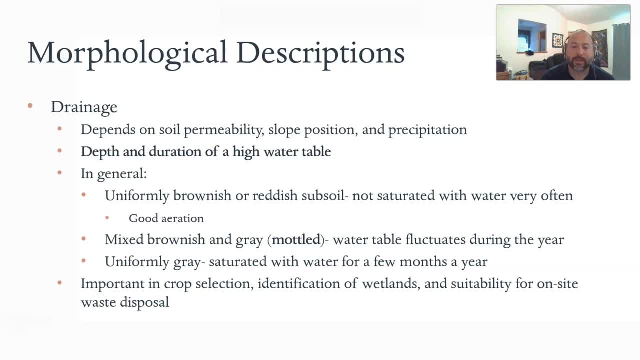 lot farther. and then there's uniformly gray, which means it's going to be saturated with water for a few months a year, and drainage is super important when we're talking about crop selection, when we're talking about trying to identify wetland areas and what's. what are certain types of? 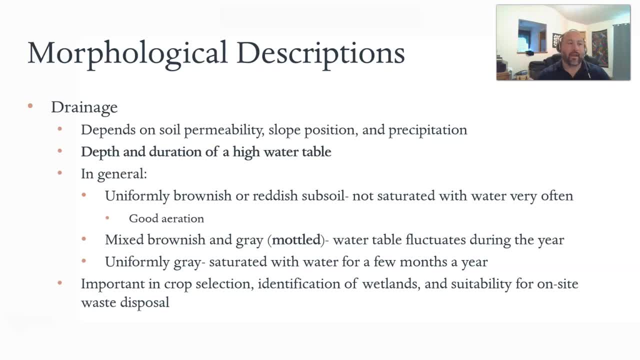 wetlands, like what's an ephemeral wetland or what's a a more permanent wetland, suitability for on-site waste disposal. if that was something we were, if we were trying to accomplish, because it's going to be important to know how wet, how wet the soil is and how water moves through the soil. 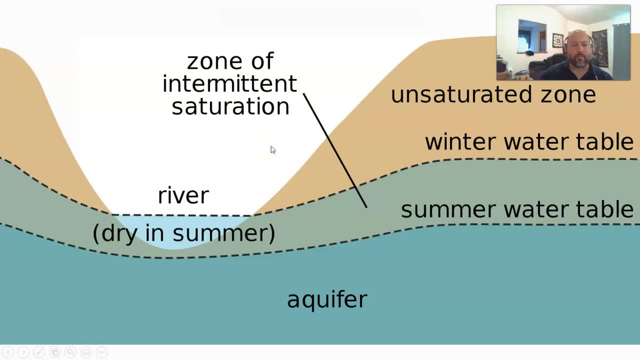 so just giving you. we'll. we'll go into detail more when we talk about soil, water relationships, but just to give you an idea of of a water table. so all we're saying when we're saying the water table is the top of wherever the water is. 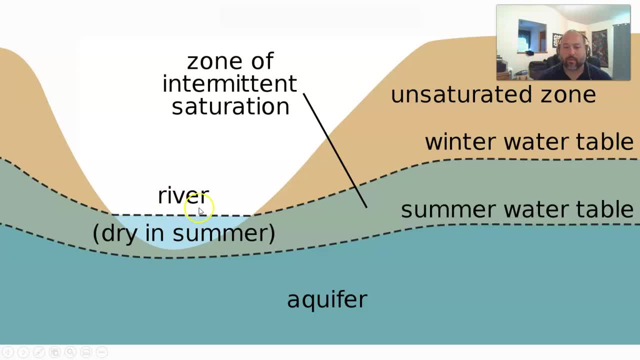 within the soil, and so if we see something like a river or a lake, all that means is the water table is above where the ground is, and that's why the water pools up on top of the ground. and so when a lot of places, what you'll see, 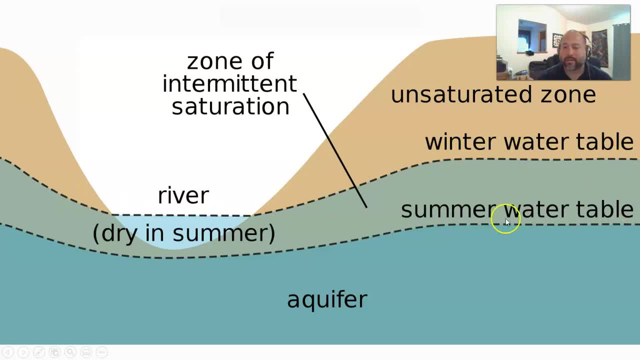 is, you'll have a higher winter water table. racism is oftenми a summer water table because you have usually, especially out here in the western United States and especially in California, we get wet winters and we get dry summers, And so you'll usually see 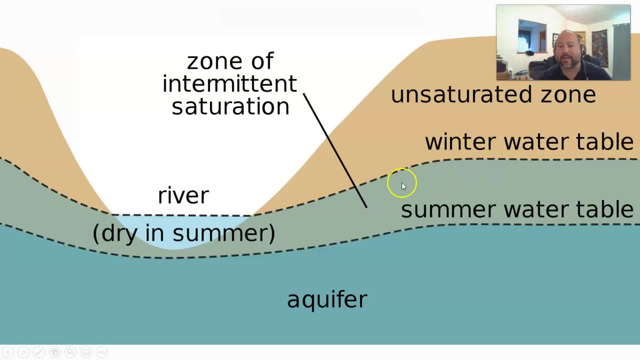 a much higher water table. It'll be much easier to dig and get to water in the winter than it will in the summer. And then, of course, down below, here is where we've got our groundwater. And then up above, here is our unsaturated zone or our vetos zone, And the reason that that is unsaturated is 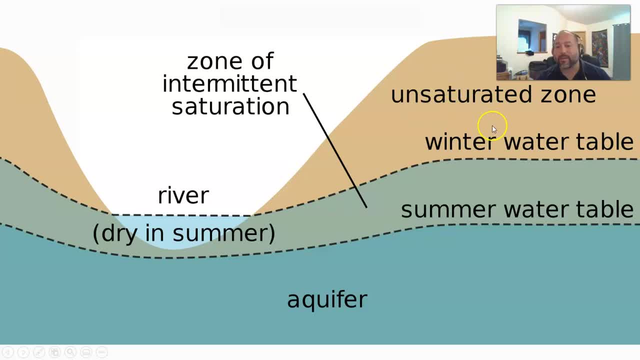 because we've got plants and we've got soil and we've got all these things that are actually using the water, And so then whatever water doesn't get used up there permeates through the soil, percolates and infiltrates and then ends up down here in the aquifer as stored groundwater. 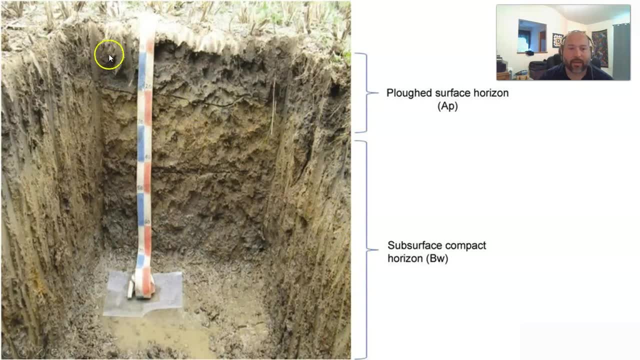 So here's kind of a look, you know, because we've been talking about this whole thing before. Here's our soil profile. We can see there's definitely different colors going on in here. So we've got a lot of different colors going on in here. So we've got a lot of different colors going on in here. 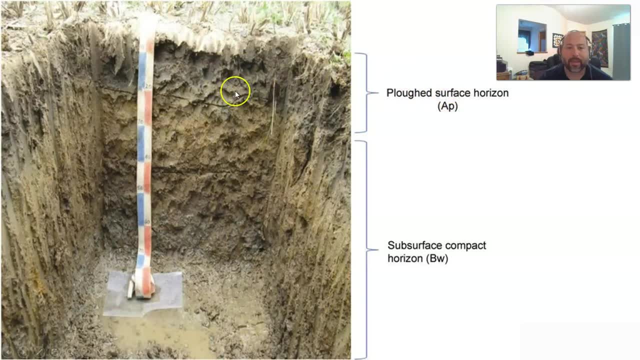 We've got a plowed surface horizon. That's an AP or it's a. it's our topsoil that's been plowed. We can see down here. we've got a BW, So we've got that changing of color happening and it's our. 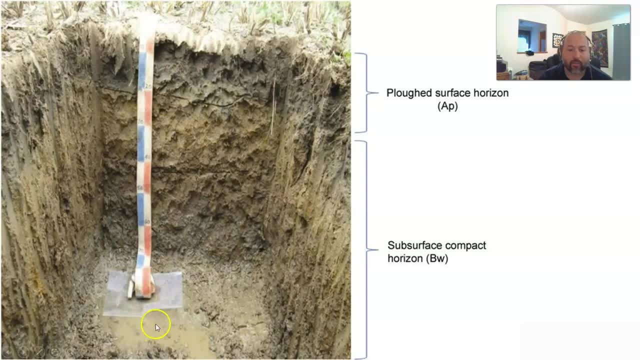 subsoil, And then we can see down here that we've hit water. So that's the water table. So if we were trying to figure out the depth of the water table, we would just measure until we got to here and that would tell us where we're at. And then we've got a lot of different colors going on in here. 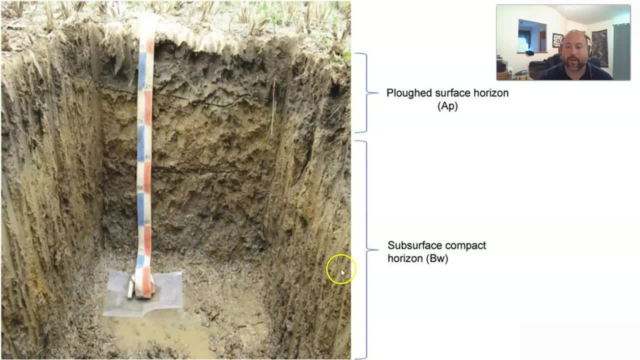 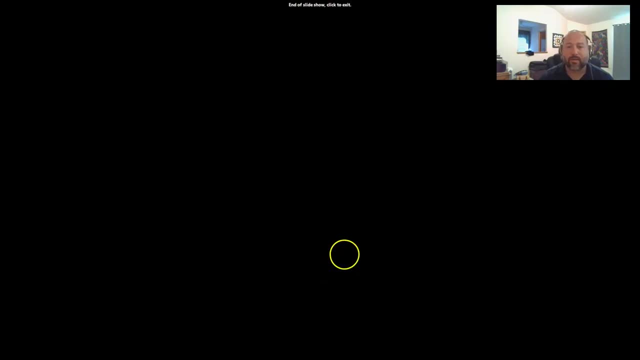 So we've got a lot of different colors going on in here. So we've got a lot of different colors going on in here. We're the start of our water is within, within the ground, And that's what I got in terms of morphological description. So I hope you enjoyed that and we'll just kind of continue on from there.